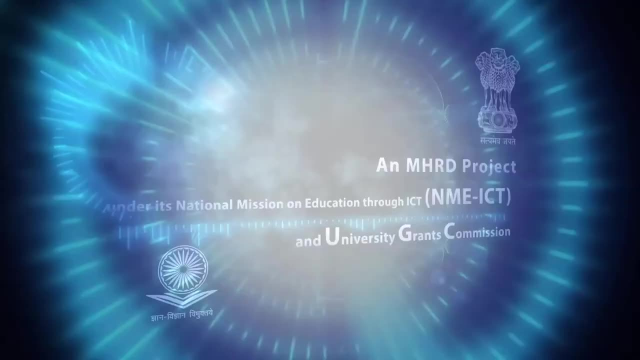 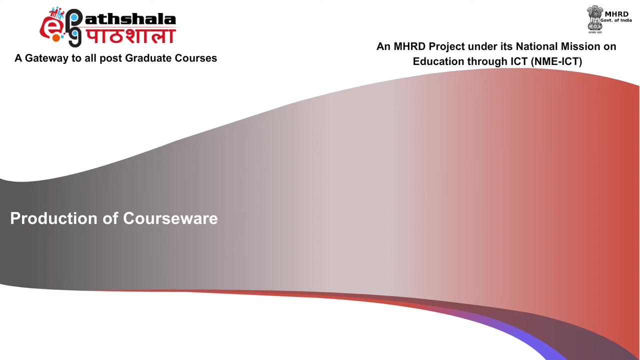 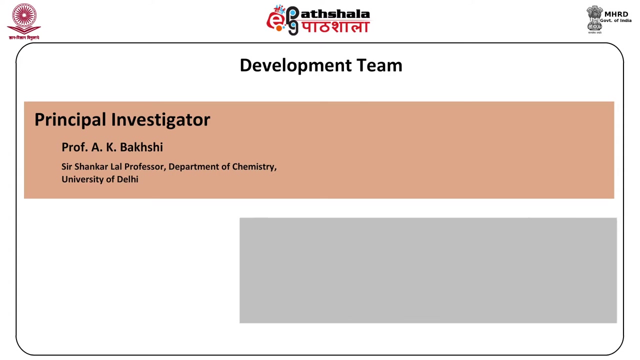 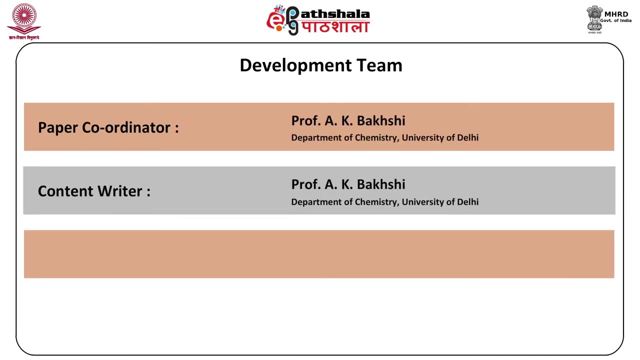 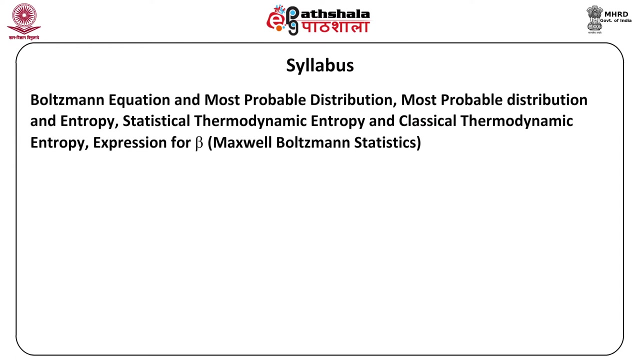 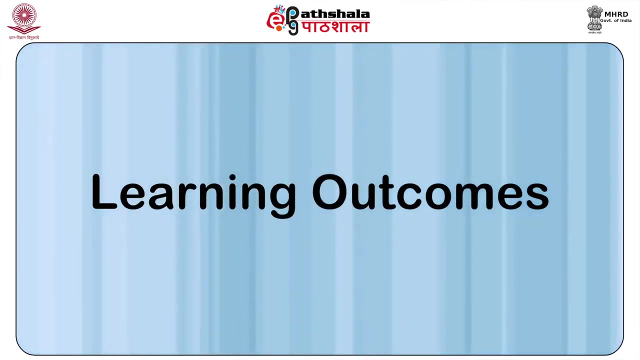 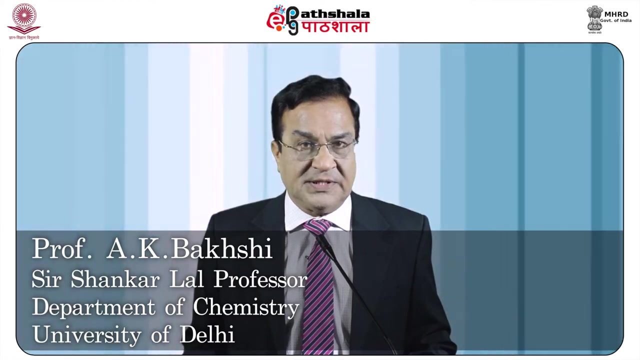 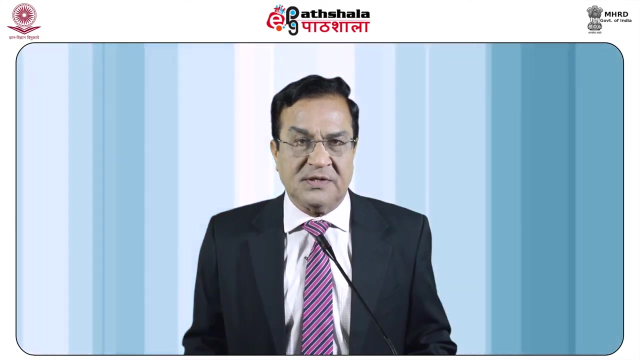 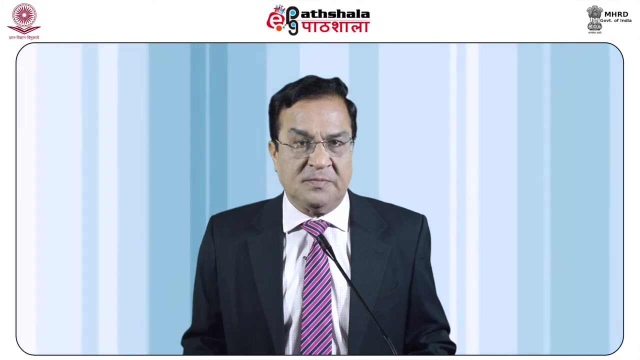 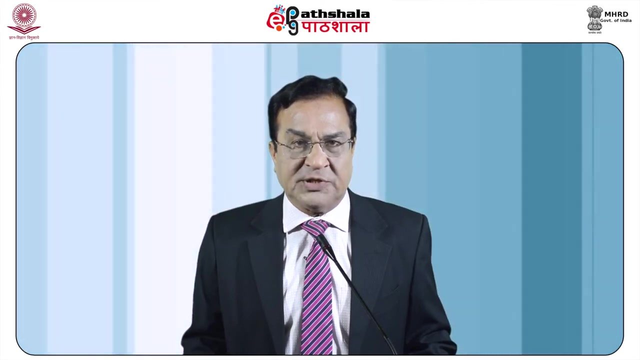 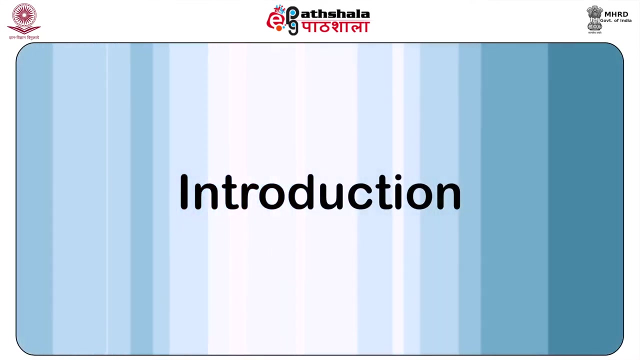 Thank you for watching. Thank you for watching. After having studied the distribution laws for all three types of statistics, in this module we will talk about Boltzmann equation, which relates bulk and microscopic behavior. We will also learn about most probable distribution And then derive the relationship between the partition function and the thermodynamic properties. 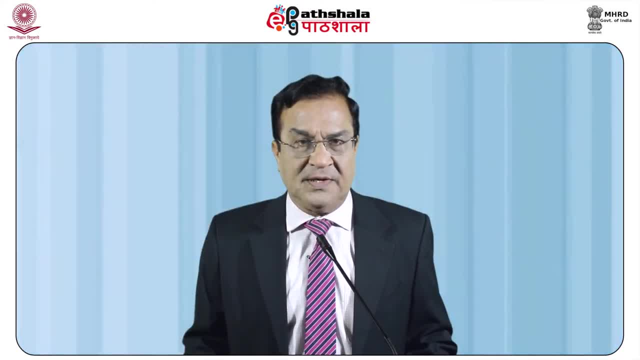 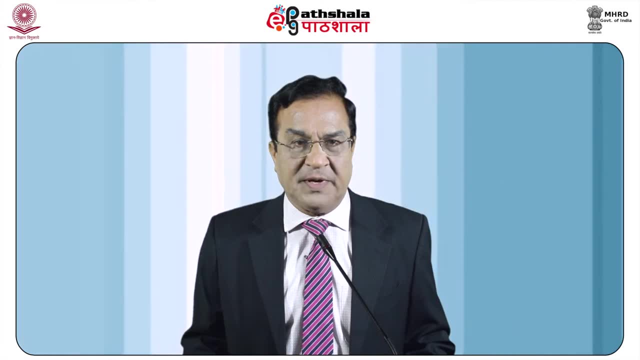 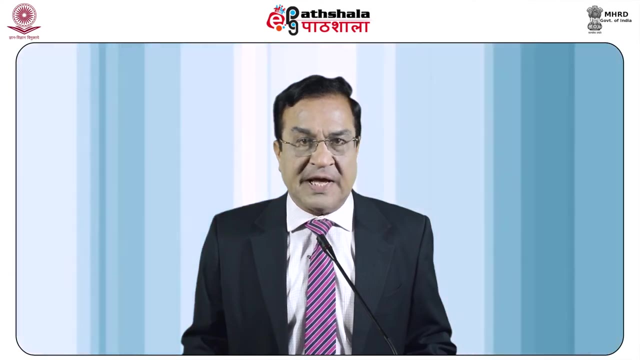 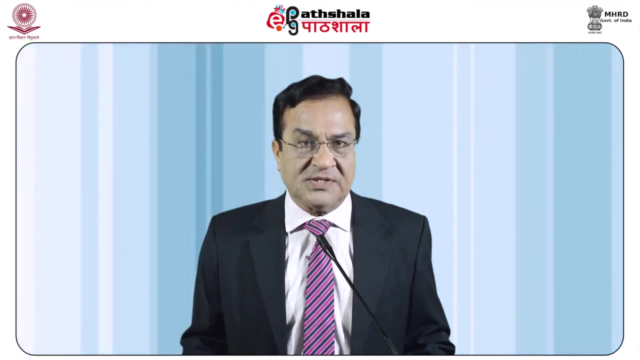 In this module we will first of all discuss how bulk thermodynamic properties are related to microscopic behavior of particles constituting a system. In the last module we talked about the variation. We have already discussed various types of statistics, which are basically classical statistics and quantum statistics. 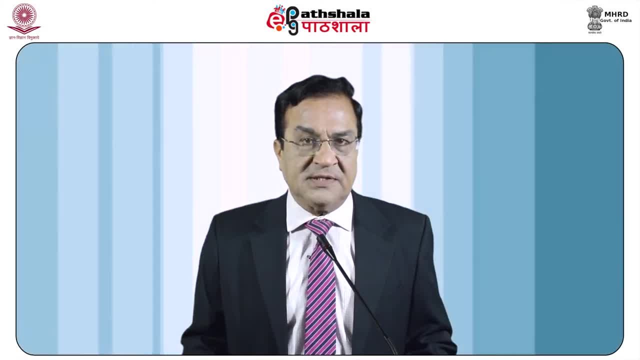 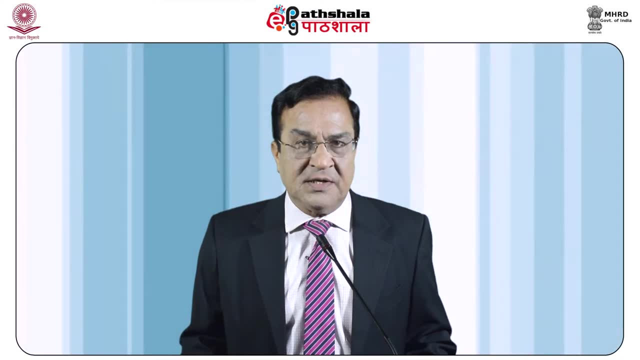 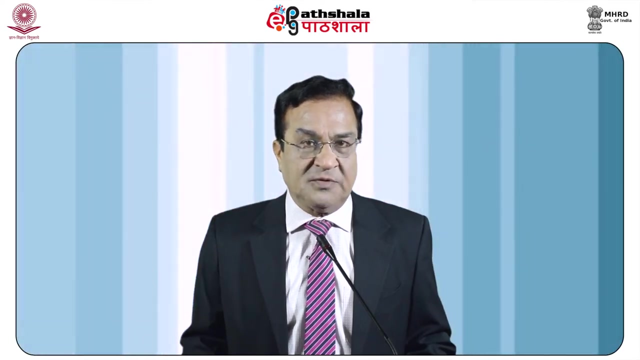 And then for each one of them we know what is the value of W for which gives the number of macro states, And then what value of NI will make W maximum. that also we have discussed in our earlier modules. We also derived last time a new expression, that is the expression for partition function. 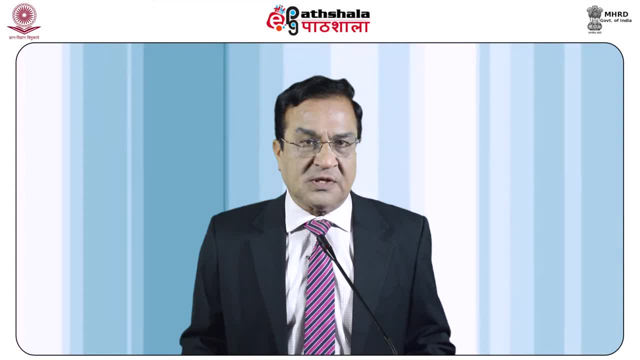 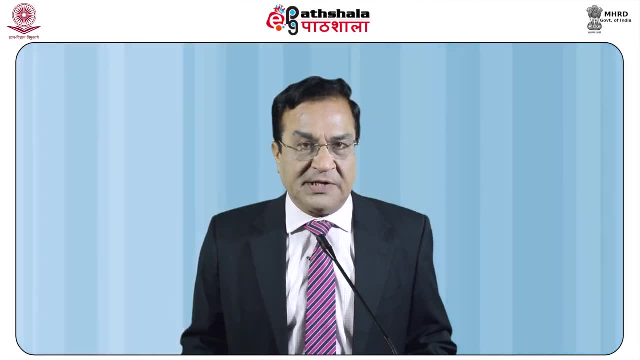 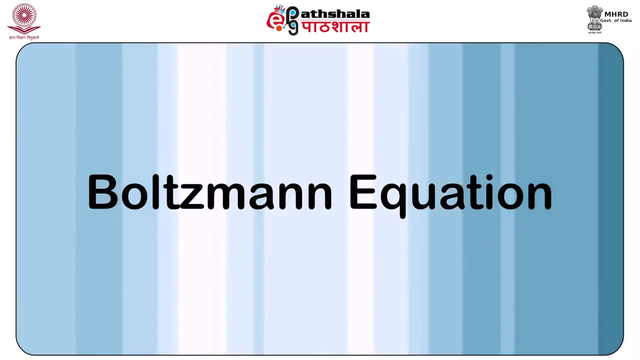 Partition function, as you know, is the storehouse of information, and all the macroscopic properties ultimately can be related to the partition function of the system. First of all, we will start with the Boltzmann equation. This is a very, very important equation of the system. 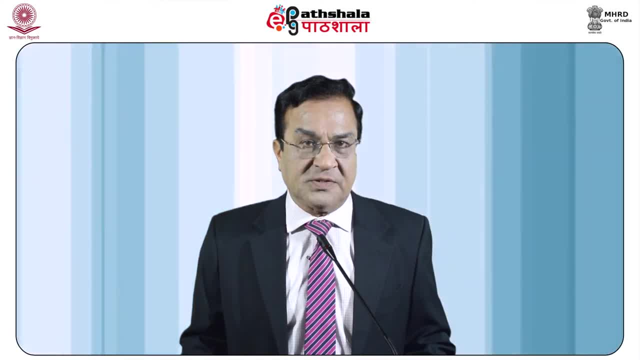 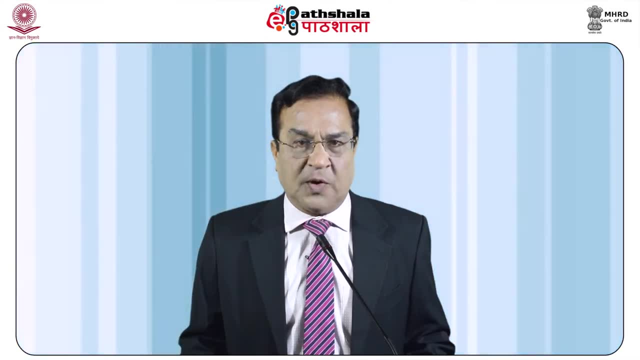 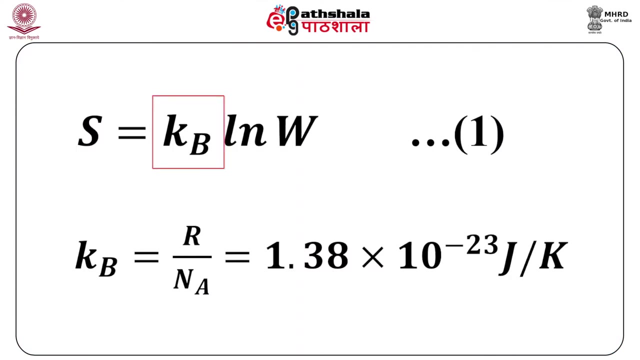 We will start with the Boltzmann equation. This is a very, very important equation of the system Statistical thermodynamics. Ludwig Boltzmann in this equation derived the formula for entropy. by giving this equation, S is equal to KB, l and W, where KB is the Boltzmann. 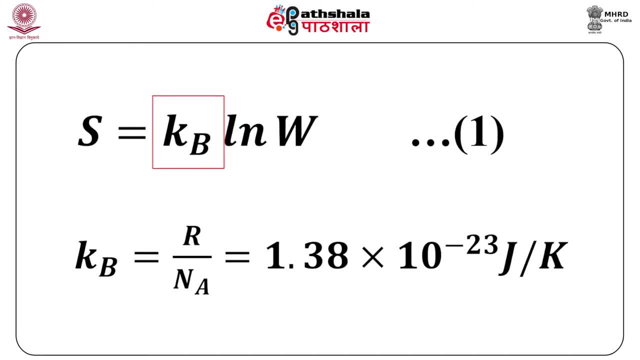 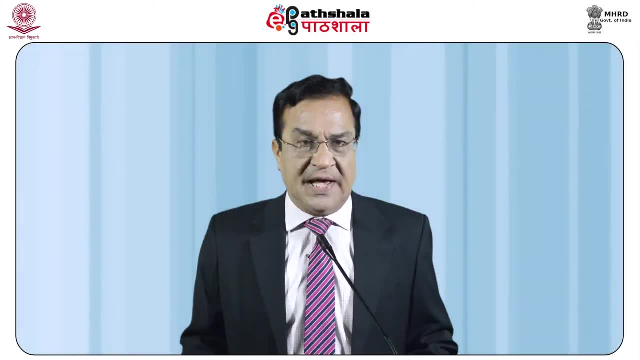 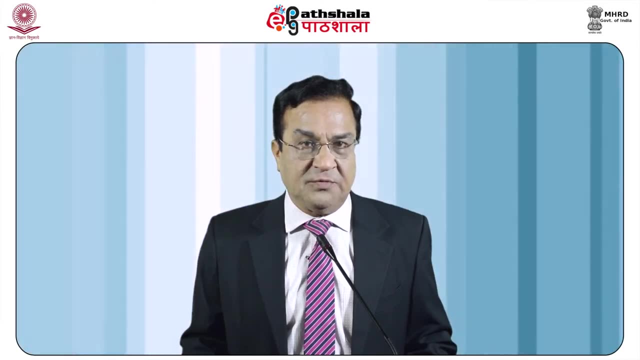 constant And its value, you all know, is 1.38 into 10 to the power minus 23 joules per K. As you can see, this equation equation is a unique type of equation. This equation has no derivation, but it is a marvelous 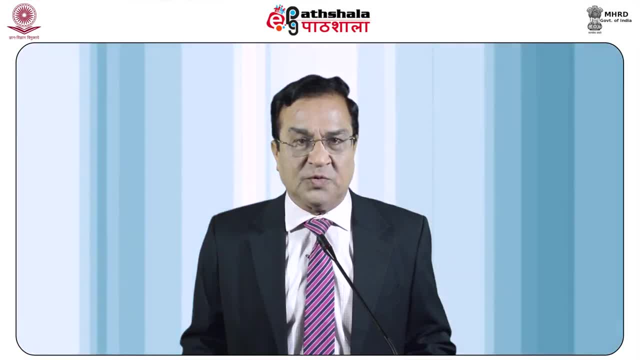 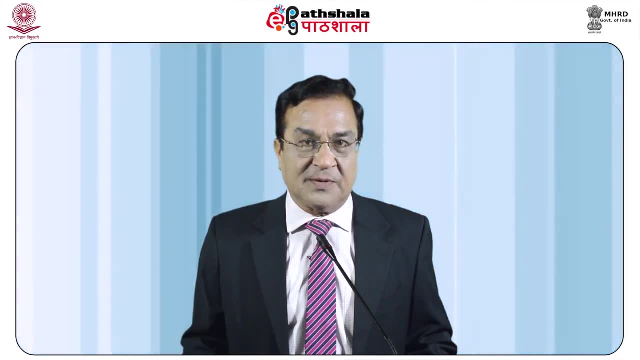 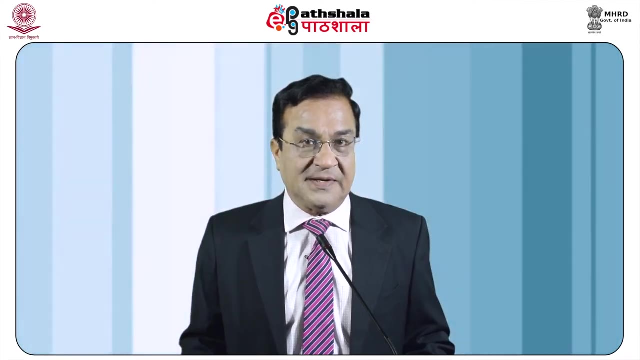 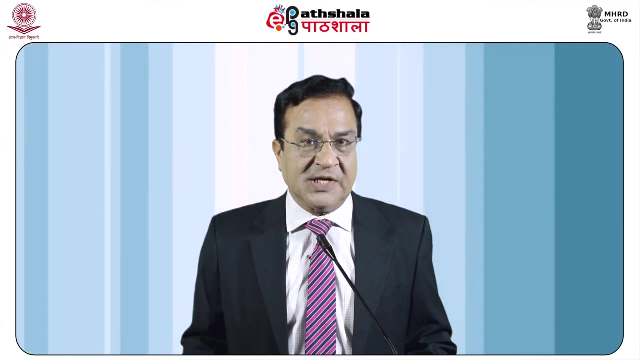 piece of contribution made by Ludwig, where a macroscopic property, entropy, which we all study in classical thermodynamics, this has been related to W, which we call as the thermodynamic probability. So it is a relationship which basically is between the bulk property, that is, entropy, and the microscopic behavior which is reflected in this equation. 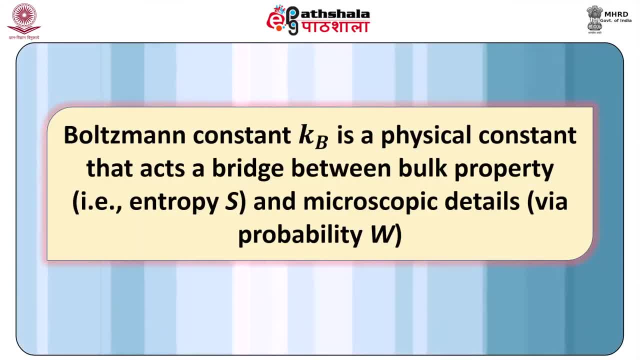 It should also be noted here that the Boltzmann constant Kb is a physical constant and it acts as a bridge between these two properties- bulk property entropy- and the microscopic thermodynamic property entropy- Probability, what we call as W. You must know that this equation forms the basis of statistical 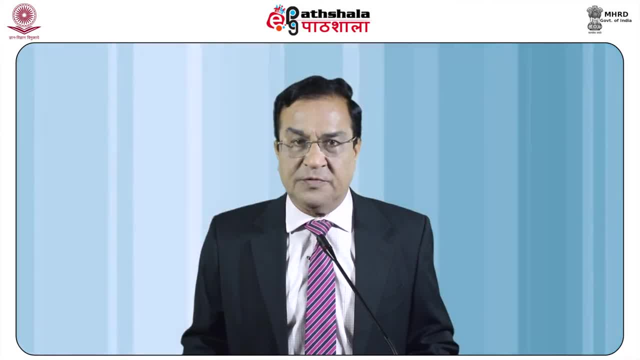 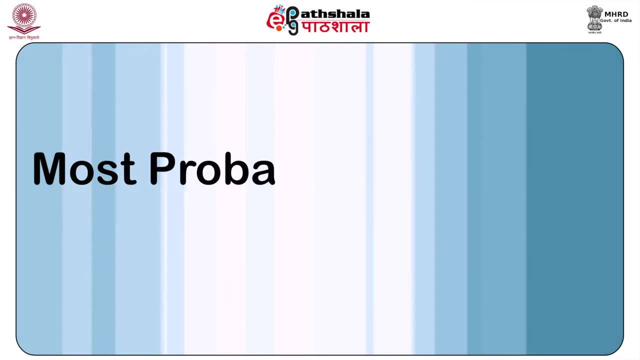 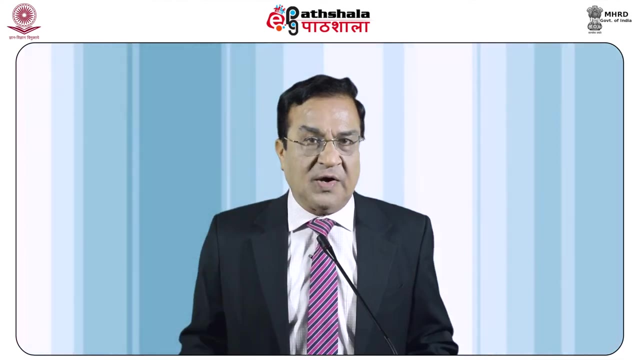 thermodynamics and for this reason Ludwig Boltzmann is referred to as the father of statistical thermodynamics. Now we will go into the details of the most probable distribution and entropy. We have already seen the Boltzmann equation which says S is equal to W. 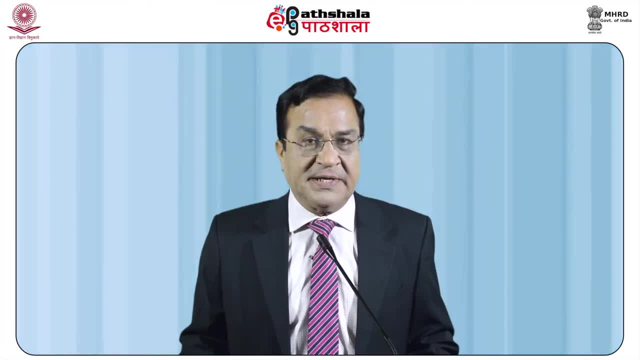 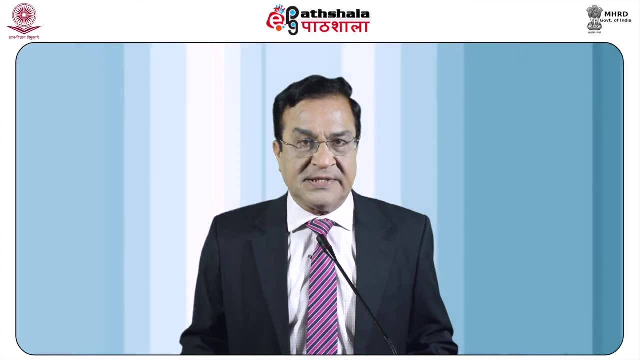 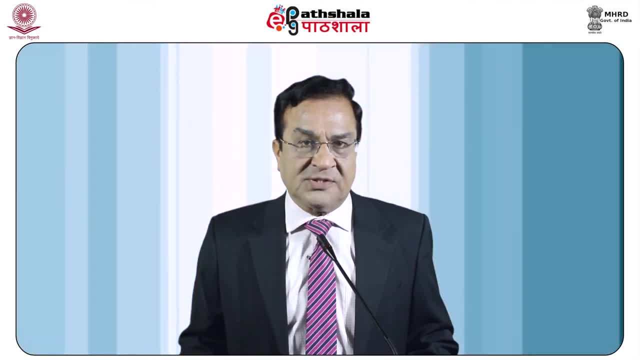 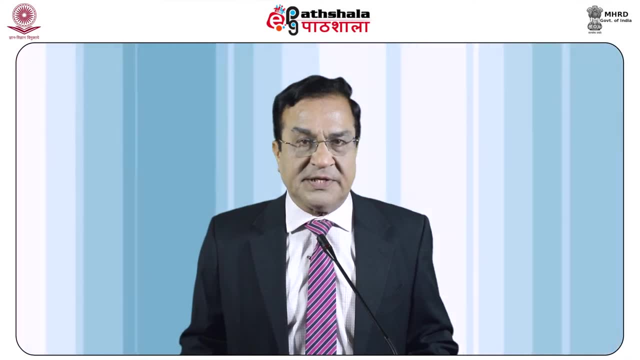 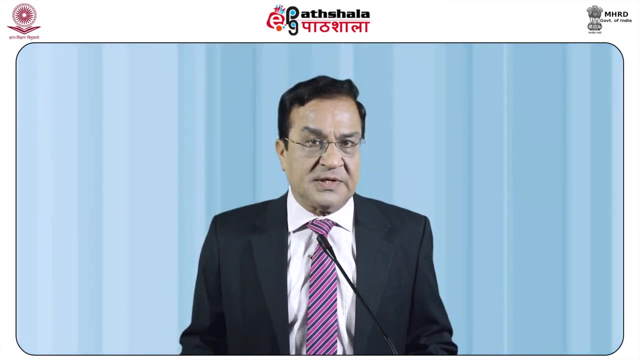 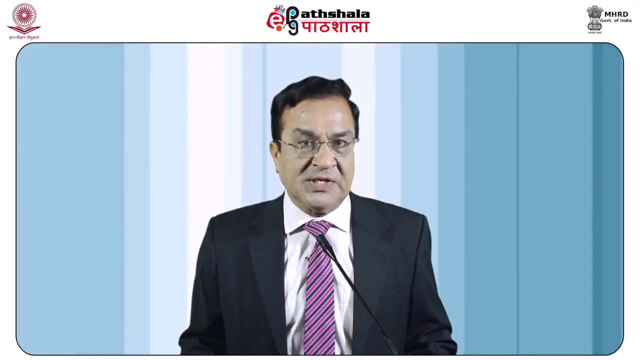 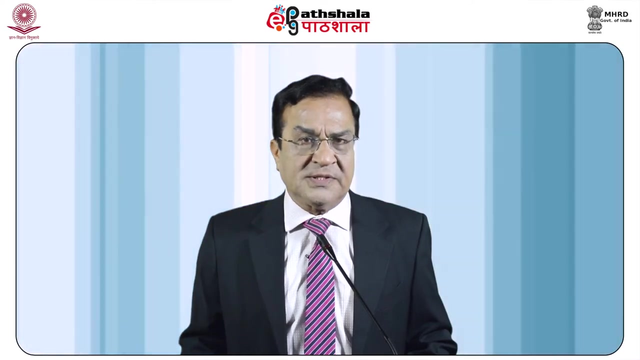 statistics we discussed that a system can have many macrostates And for each macrostate, because of the distinguishability of the particles, many microstates are possible And we also in our last module showed that which particular distribution will give the maximum value of W and that is called the most probable macrostate. Suppose a system: 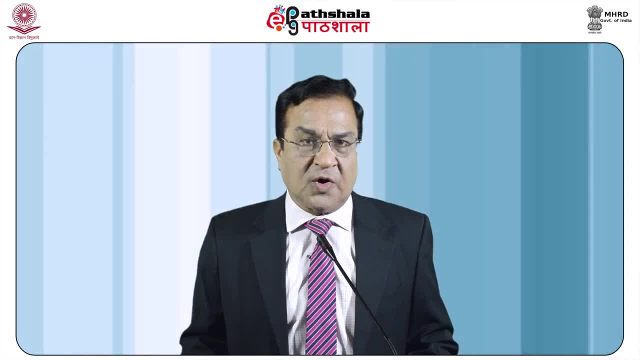 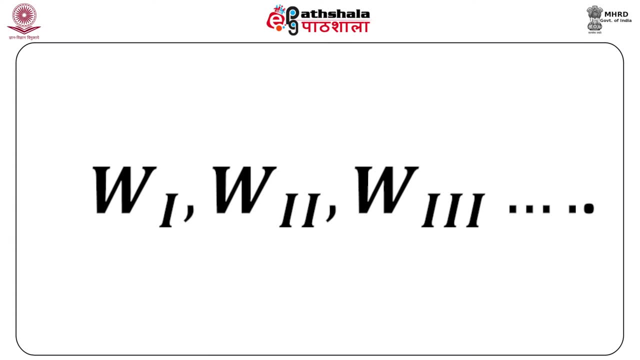 has many macrostates and then the corresponding possible microstates are W1, W2, W3, etc. And suppose we take W1, W2, W3, etc. And suppose we take W1,, W2, W3, etc. And suppose we take: 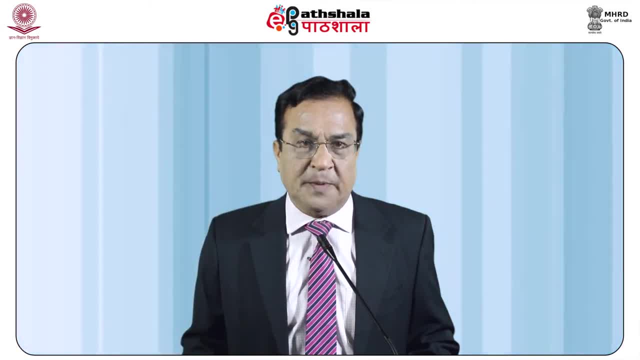 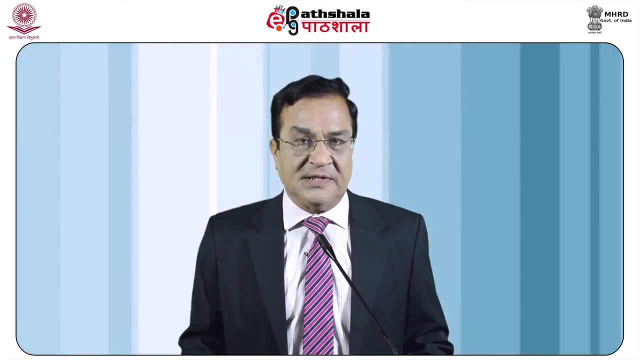 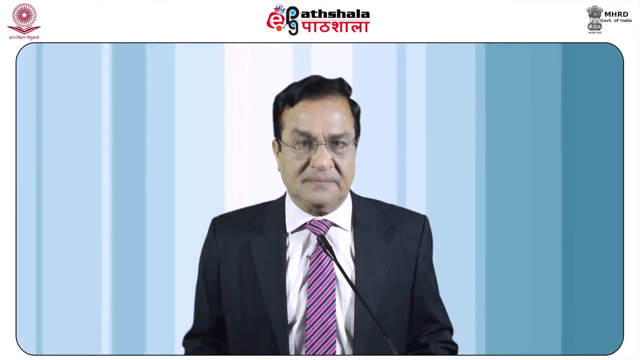 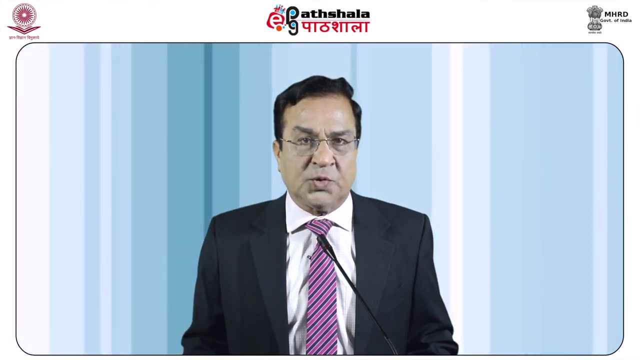 that W2 is the most probable macrostate. that means W2 as having the maximum value, or in this macrostate the number of microstates is maximum, and so we call it Wmp. And since all microstates of a system are equally probable, therefore the total number of microstates 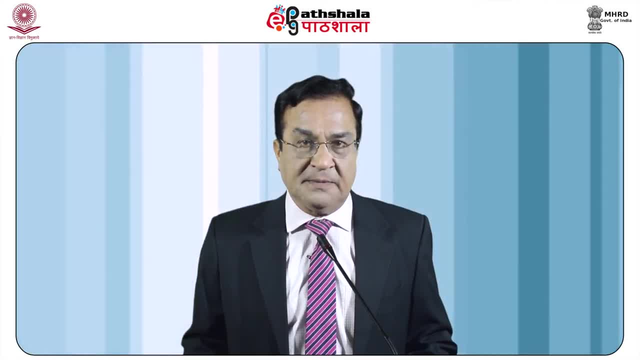 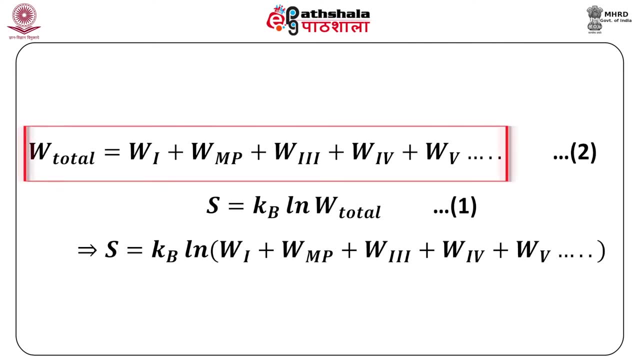 which will exist for a system is equal to Wmp. So the total number of microstates which are equally probable at a particular temperature is given by W. total equals W1 plus Wmp. Wmp is the most probable macrostate, plus W3 plus. 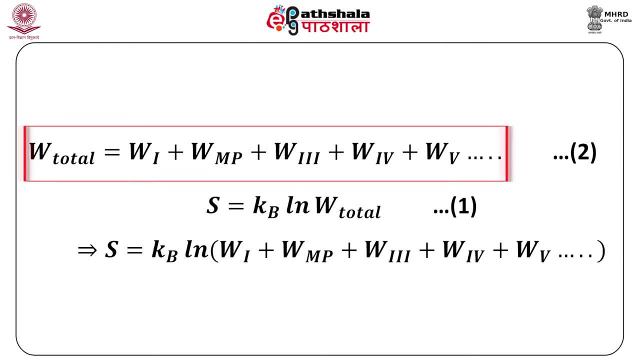 W4 plus W5 and so on. So this gives us the total number of microstates associated with that system. Now, according to our Boltzmann equation, S is equal to Kb, ln, W. Now suppose Instead of W we put W, total, that means the total number of microstates associated with. 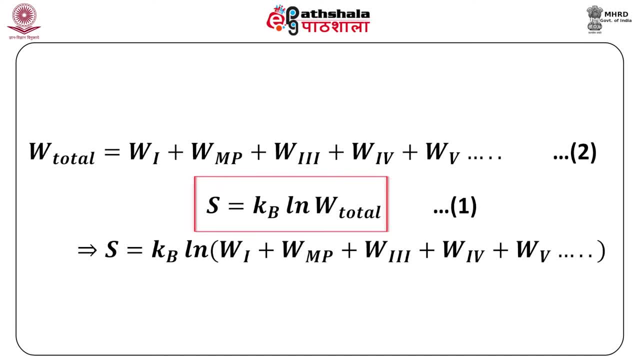 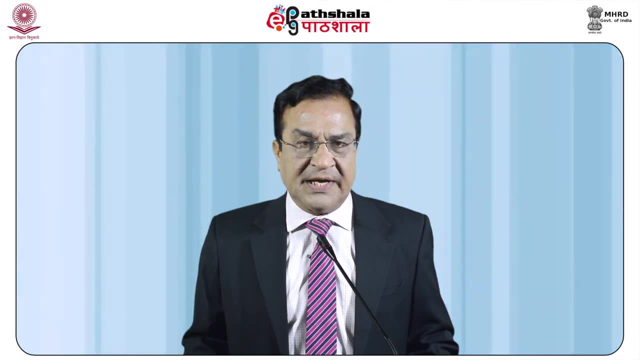 the system. Then we have, as you can see here, S is equal to Kb ln. in parenthesis we have W1 plus Wmp, plus W3 plus W4 and so on. If we rearrange, then this equation can be written as: S is equal to Kb ln, Wmp, Wmp, we. 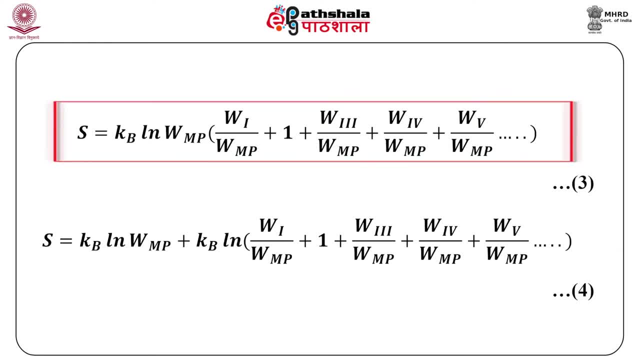 have taken out. So inside we will have W1 by Wmp plus 1 plus W3 by Wmp, and so on. Now, since Wmp has the maximum value, we have said already this- because this is the most probable microstate. So this is the number of microstates associated with the most probable microstate. 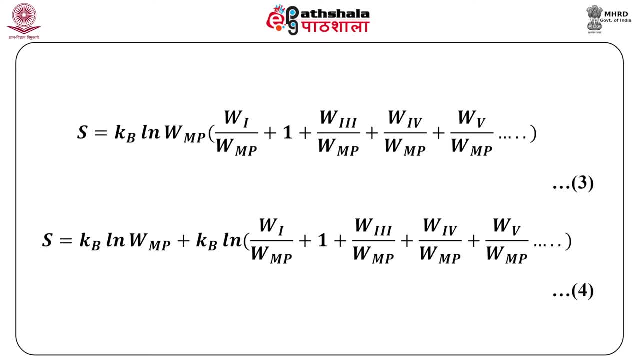 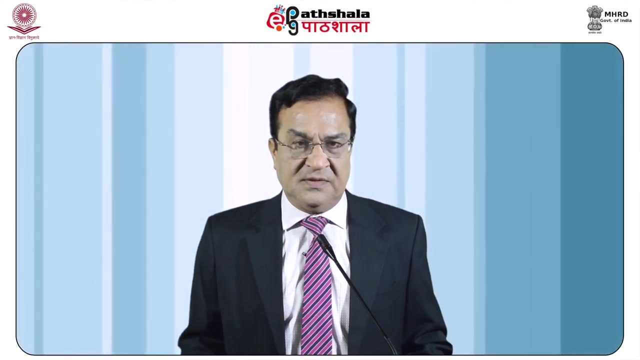 Therefore one can very easily split this equation on the right hand side into two parts. First will be: S is equal to Kb, ln Wmp plus Kb, then ln W1 by Wmp plus 1 plus W3 by Wmp, and so on. If you look at the expression in the parenthesis you can see that it will have very, very low. 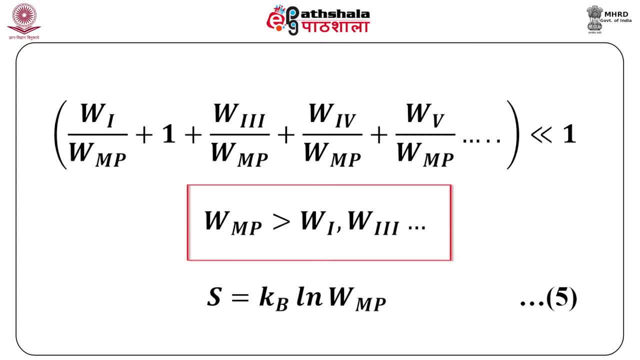 value, Because Wmp is much, much greater than W1 or W3. Hence the natural logarithm term will become very, very small And therefore you can say that we can neglect the second term. And once we neglect the second term, the equation reduces to: S is equal to Kb, ln, Wmp. 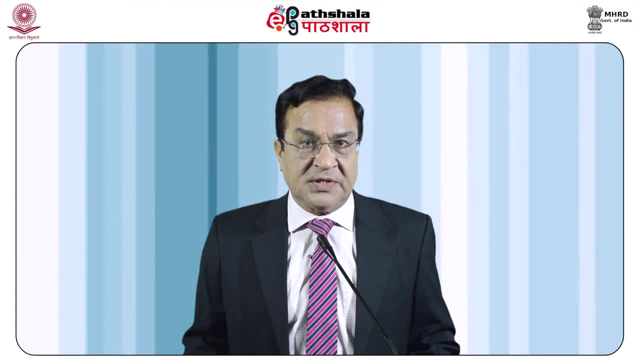 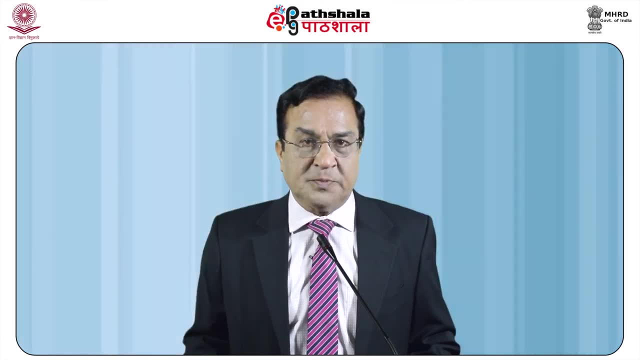 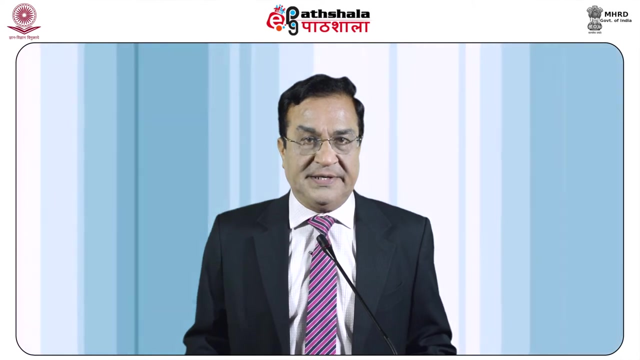 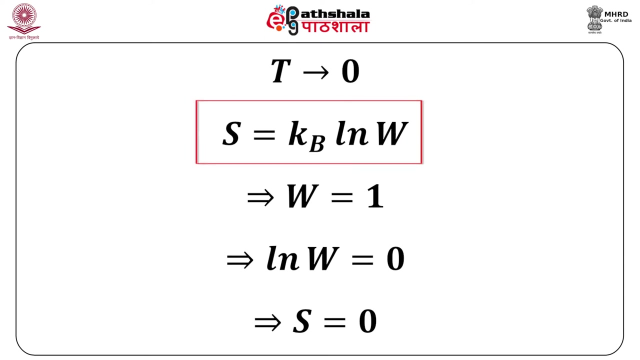 That means in Boltzmann equation we are justified in relating entropy- I am again repeating- is the number of microstates associated with the most probable microstate, and it is also called thermodynamic probability. From what we have derived now that S is equal to Kb, ln, Wmp. it means entropy which we all 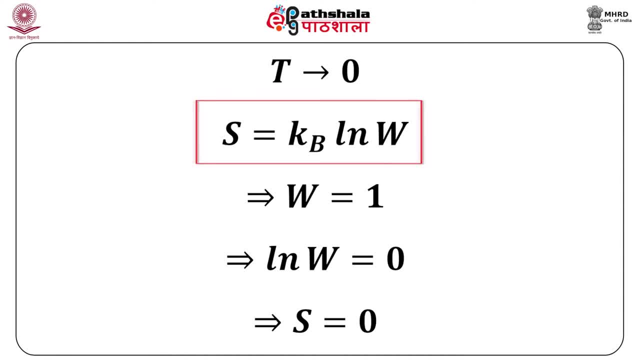 know is a measure of disorder. This is directly related to Wmp, the thermodynamic probability, and we also know that with decrease in temperature entropy decreases. So from this equation it will mean that Wmp will decrease. That means that number will decrease. 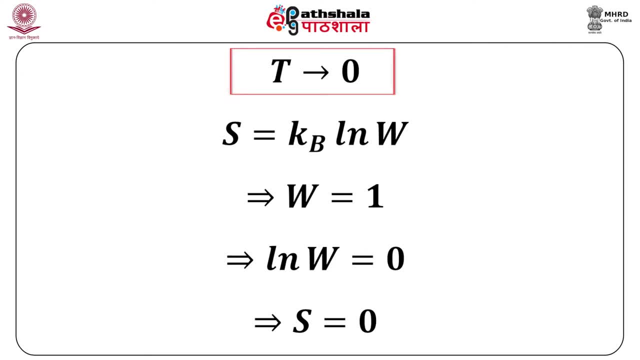 And if we keep on decreasing the temperature? suppose we reach the temperature zero absolute. in that case the corresponding entropy will become 0. and if the entropy is to become 0, then Wmp must be equal to 1.. That means there will be only one microstate associated with the most probable macrostate. 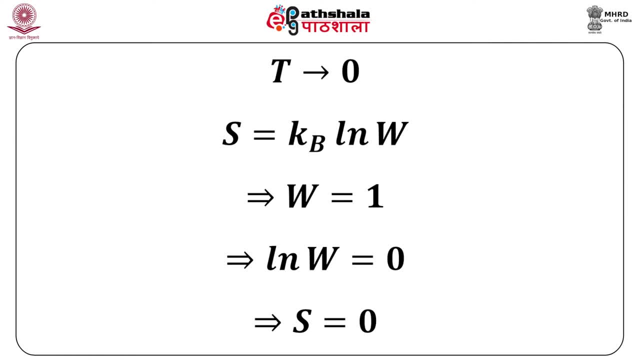 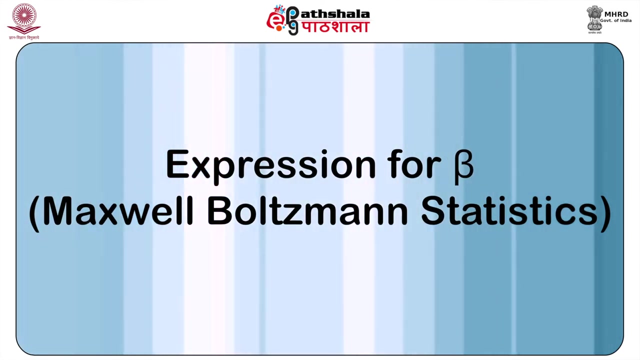 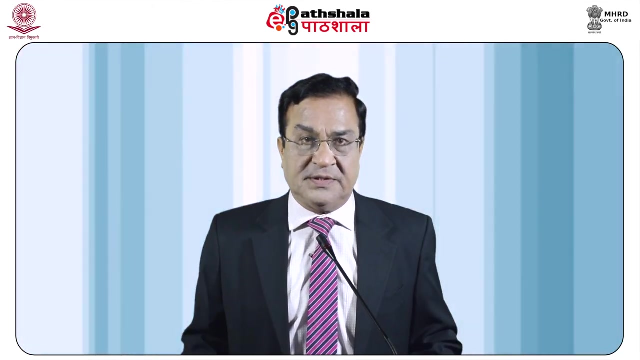 at temperature 0 absolute. So this is also what we learn from third law of thermodynamics. Third law of thermodynamics basically starts with the fact that for any crystalline solid at 0K, the entropy is 0.. After having said all this now we will move further. 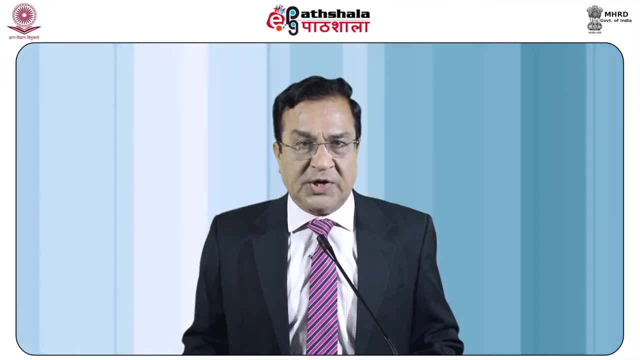 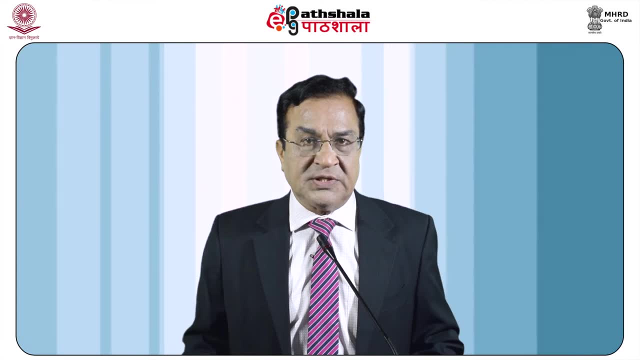 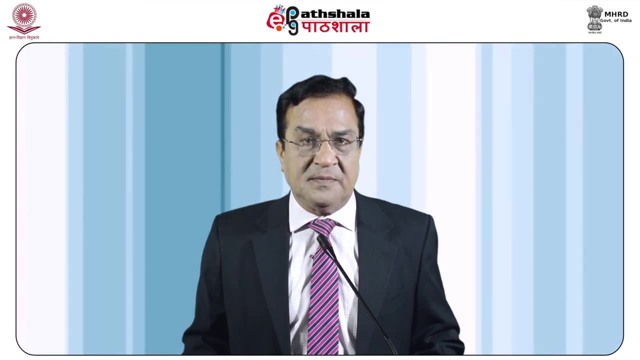 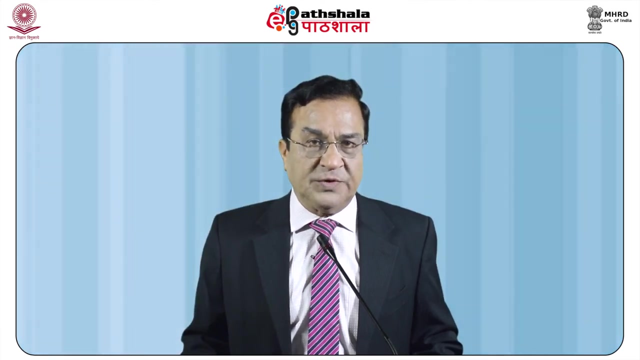 You remember that in the last module we talked about partition function And we said that partition function Q is given by the relation summation Gi, e to the power β, epsilon i. But we do not know yet what is the value of β, although we said that it will be shown. 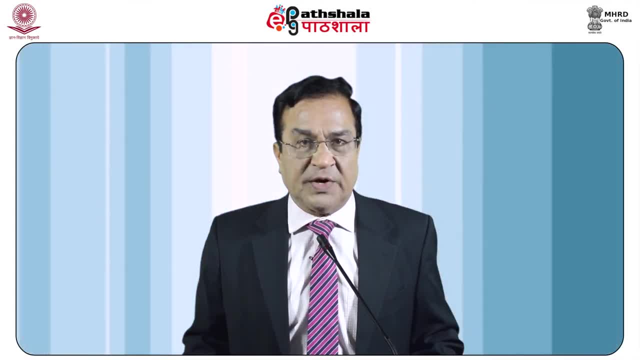 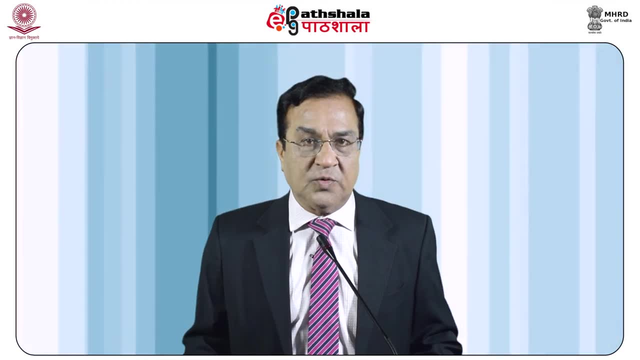 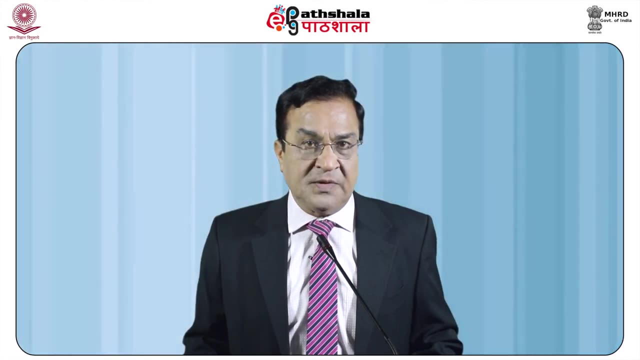 later on that β is equal to minus 1 upon kT. So today we will discuss this and show how β comes out to be equal to minus 1 upon kT. We have already studied that if we have a system consisting of n particles and having 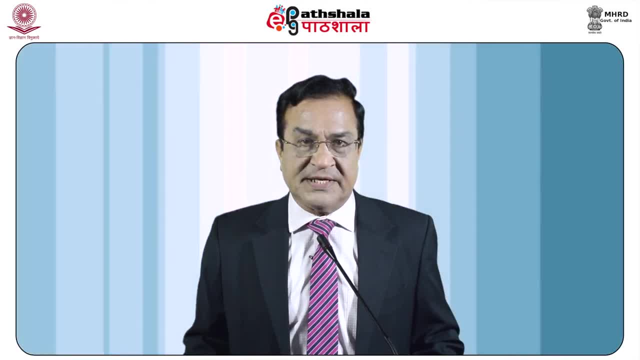 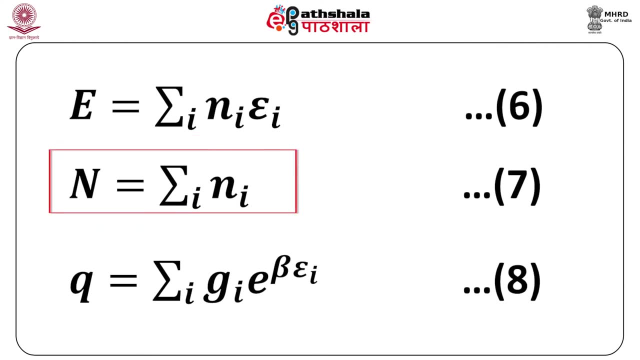 total energy, E. obeying Maxwell Boltzmann statistics, then E is equal to summation i ni epsilon i And capital N. that means the number of particles is equal to summation i ni, where we all know that N refers to the total number of particles. 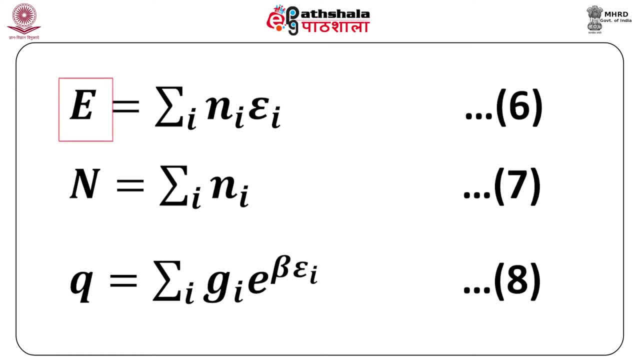 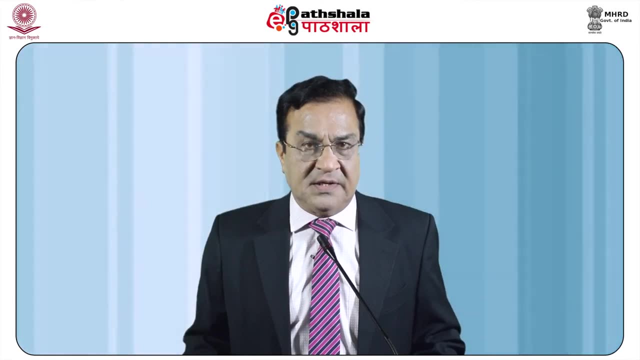 And E is the number of particles, The total energy of the system. Now the partition function, as we just now mentioned, is summation: i Gi e to the power, β epsilon i. And we also know that for the most probable macro state, if we have to find out, W is given. 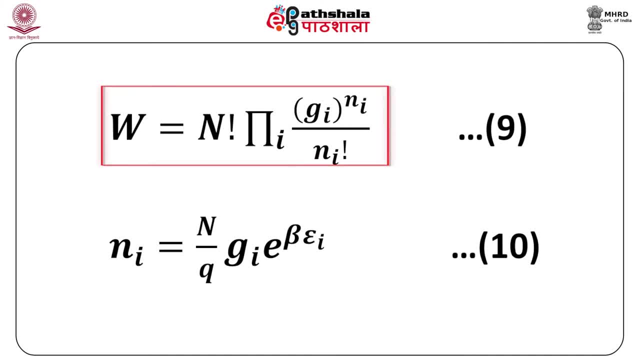 by N factorial. pi i Gi raise to the power ni upon ni factorial, But for most probable distribution small ni is given by N factorial. So this is the total energy of the system. Now the partition function, as we just now mentioned, is summation. i Gi e to the power. 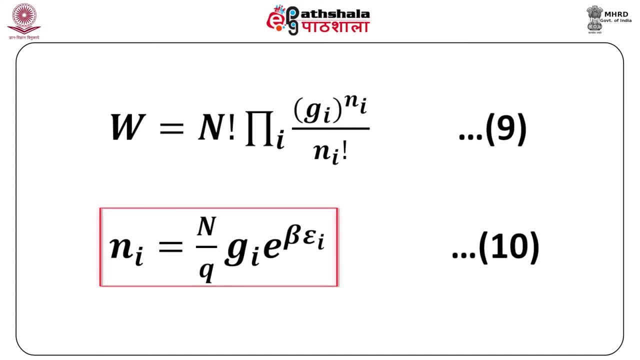 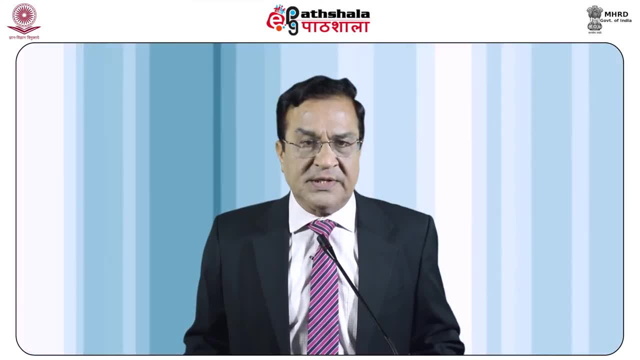 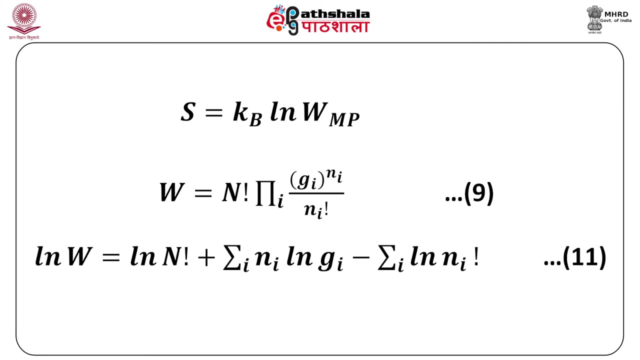 beta, epsilon i. All these equations we have already learned. Now what we will do is we will discuss further and calculate entropy expression from this. We have already shown that S is equal to Kb, ln, Wmp. Now, taking natural logarithm of this, is our equation 9.. 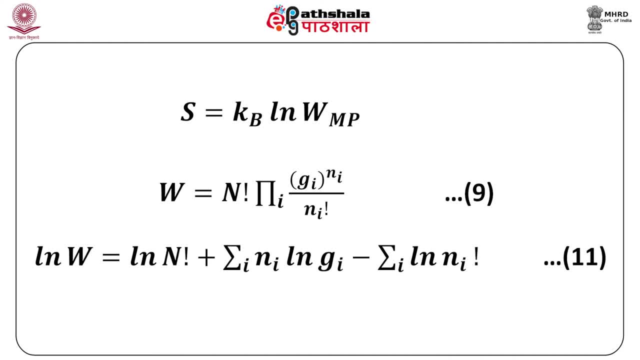 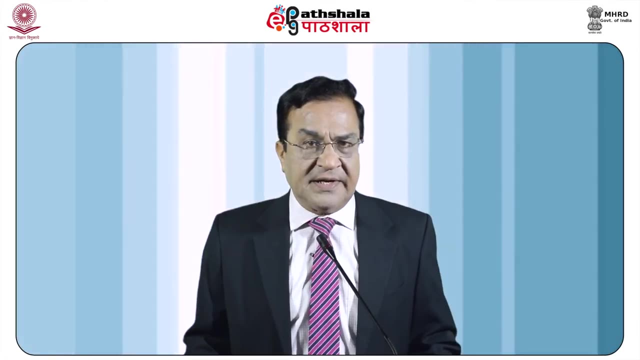 If we take logarithm of this, This becomes Sb. ln W becomes equal to ln N factorial. summation i ni ln Gi minus summation i ln ni factorial. Please notice here that we have removed the symbol mp now, because in general we will be. 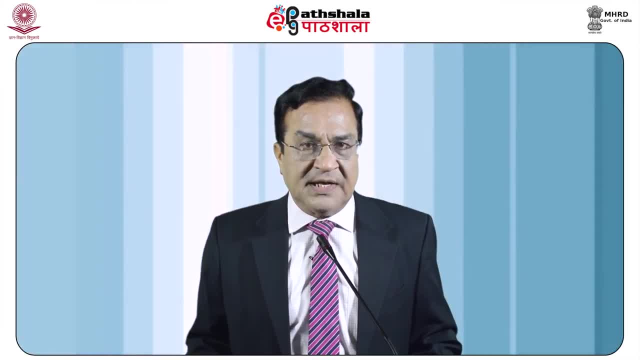 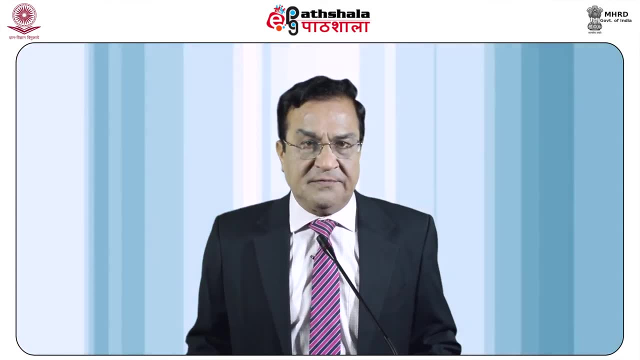 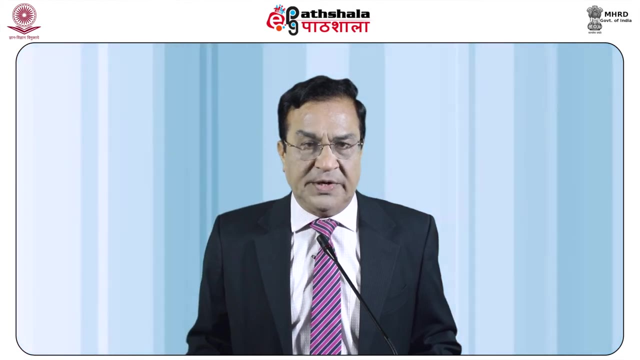 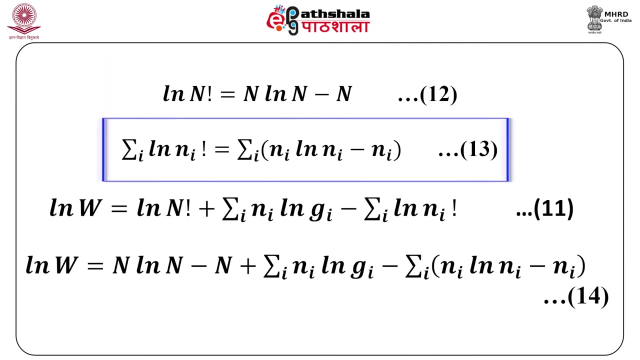 talking about W and W will always in this equation, will refer to the most probable macro state. Now, once we have this equation, now we can apply sterling approximation and simplify it further. We know what is the sterling approximation: ln N factorial is equal to n, ln N minus N. 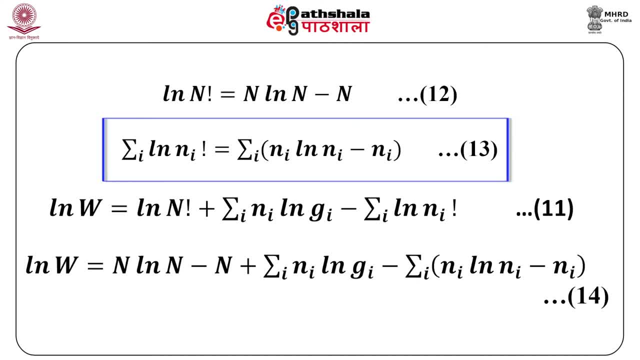 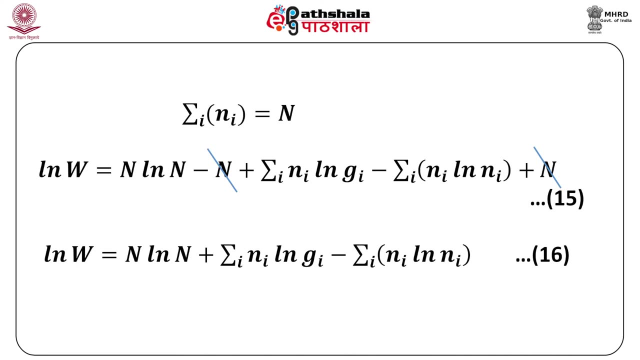 and similarly for ln ni factorial. also, we have the sterling approximation. So if we substitute these values in the expression for ln W And simplify it as see we have done it here, ultimately we will get: ln W is equal to n ln N plus summation i ni ln Gi, minus summation i ni ln Ni. that is the equation 16 which we 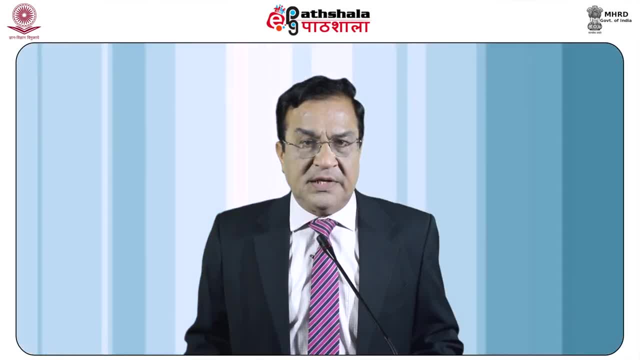 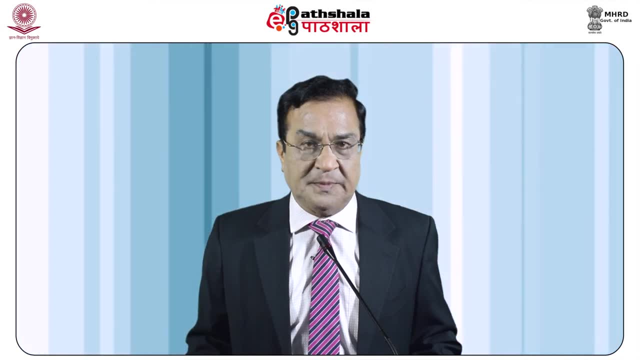 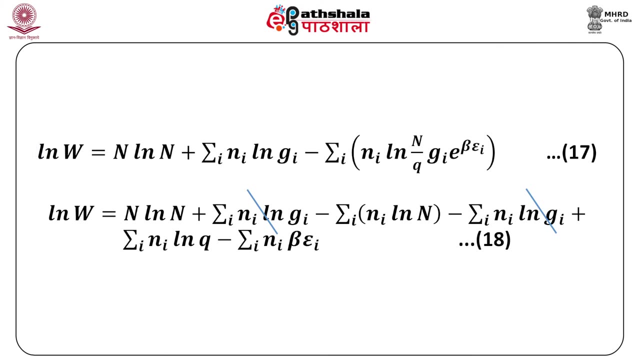 have got. And now, if in this equation we substitute the value of ni, The value of Ni, The value of Ni, Which comes for the most probable distribution, we have the equation 17. as you can see, Here we have substituted the value of Ni. 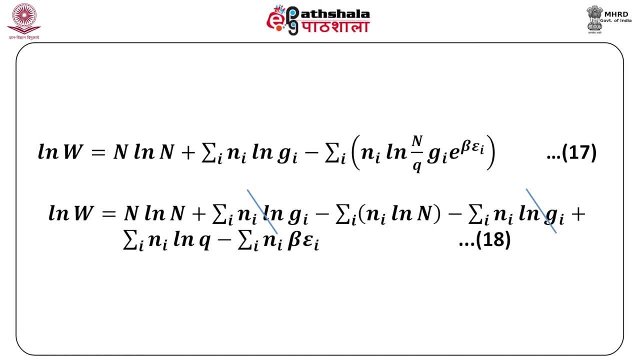 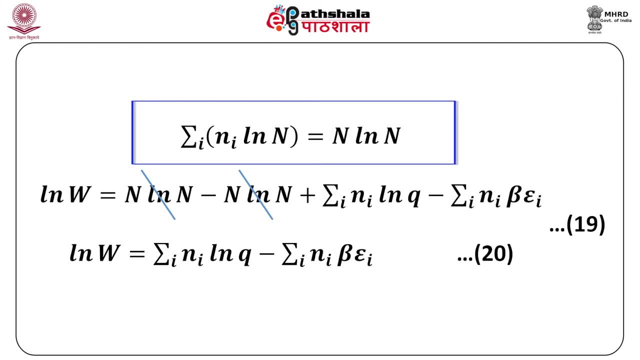 We have substituted it only in the last part, as you can see here, And if we simplify it and use this relation, that summation i ni ln N will be equal to n ln N. One notices that ultimately we get the value of Ni. Okay, 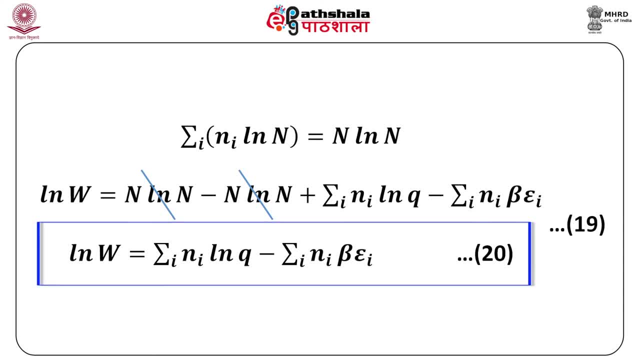 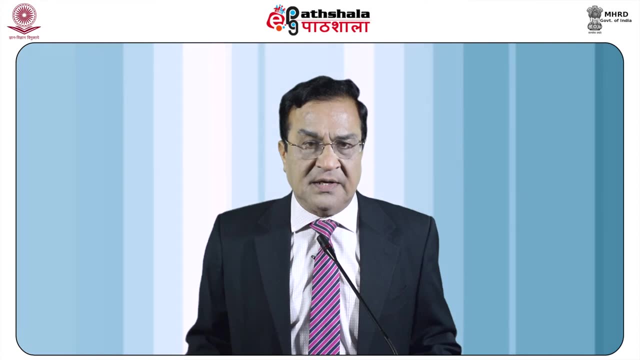 We get: ln W is equal to n, ln Q minus beta E. So this is a very, very important equation. Here capital N is, of course, the number of the particles. Q is the partition function. beta is something which we introduced earlier in the Lagrange's method of undetermined. 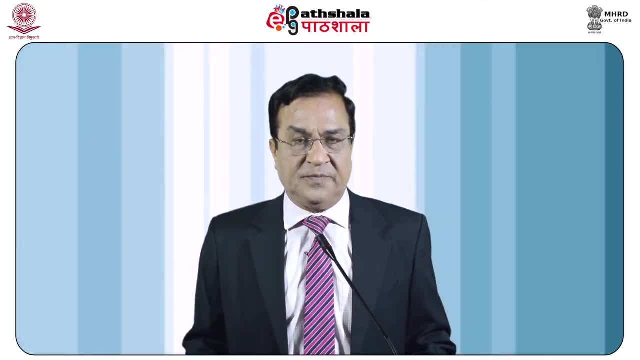 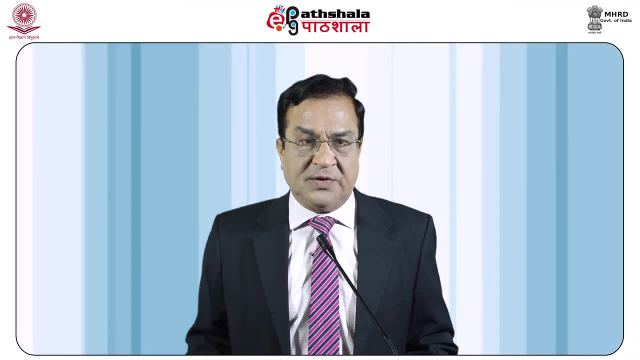 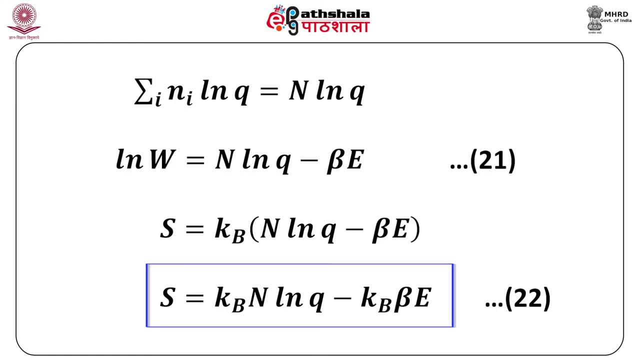 multipliers and E is the total energy of the system. Now if we substitute this expression, If we substitute this expression of ln W in Boltzmann equation, we get the equation as you can see here. S is equal to kB N, ln Q minus kB beta E. So this is a very important relation. 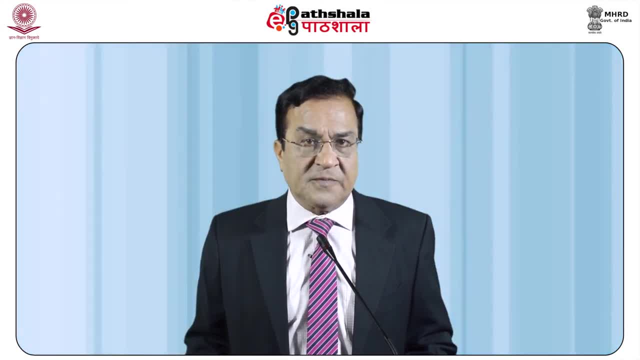 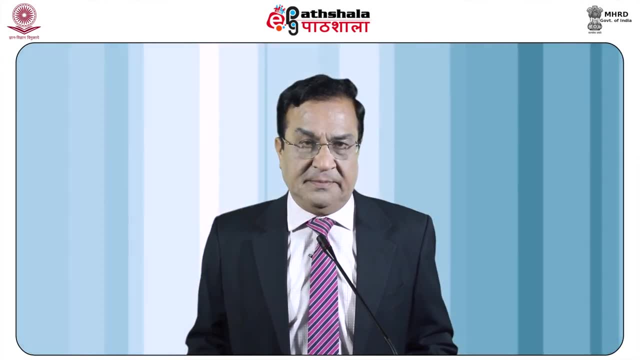 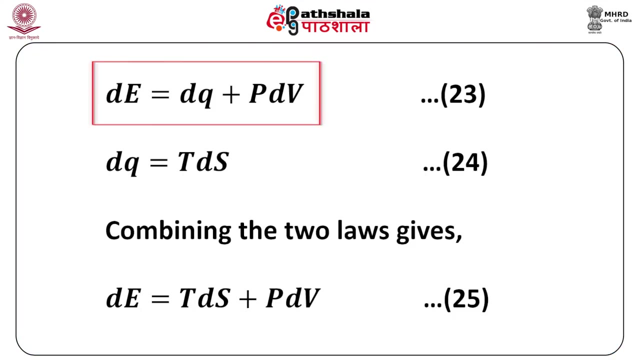 But our aim is still to find out the value of beta. now we will do that. we already have studied in classical thermodynamics. Okay, I am sure you all must be familiar with this first law of thermodynamics definition, which is: dE is equal to dQ plus PdV. and then second law of thermodynamics gives us the definition. 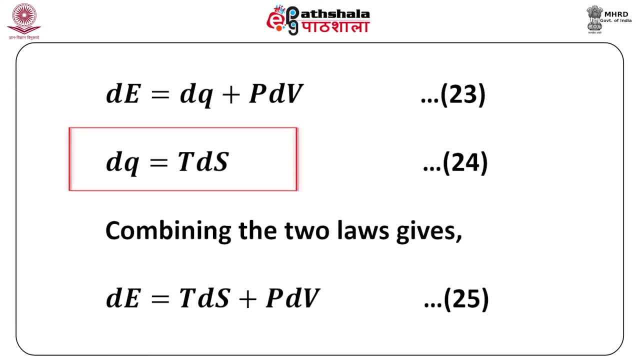 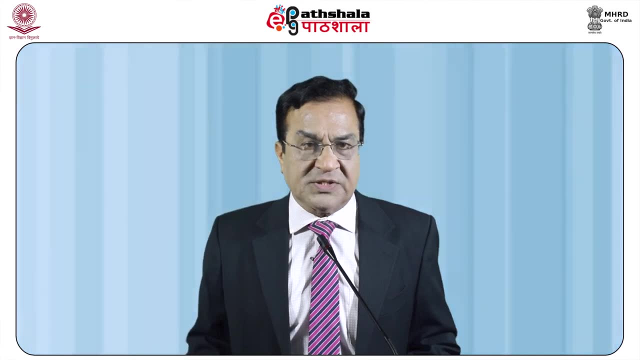 of entropy, and that is dQ is equal to TdS. If we combine these two laws, we get dE is equal to TdS plus PdV. and if we differentiate this equation With respect to E at constant volume, we get this equation which further reduces to as: 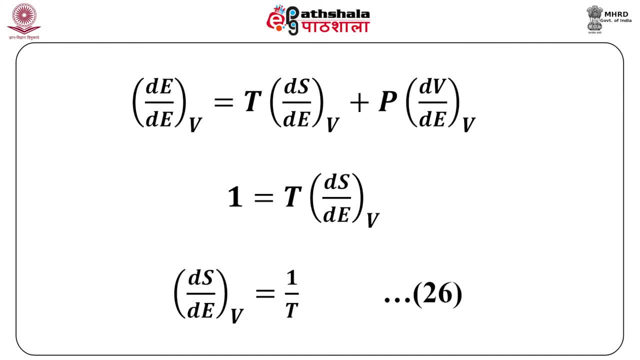 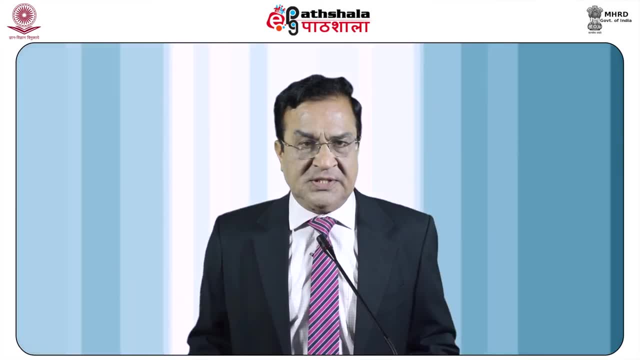 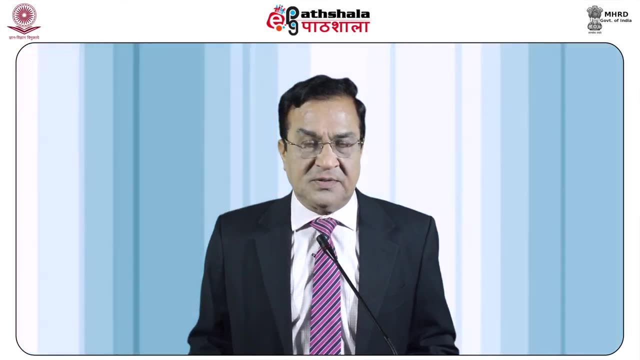 you can see, ultimately we get dS by dE at constant volume is equal to 1 upon temperature. So this is basically coming by the combination of first and second laws of thermodynamics. So this is basically comes from classical thermodynamics. 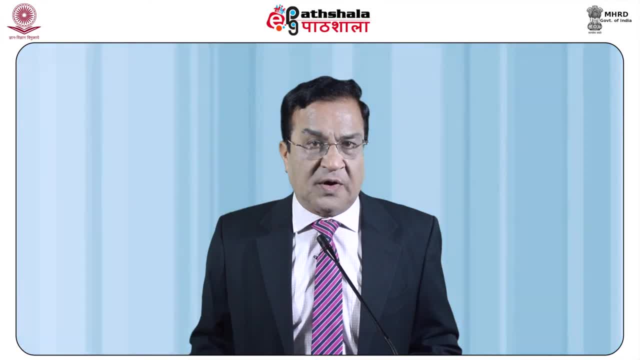 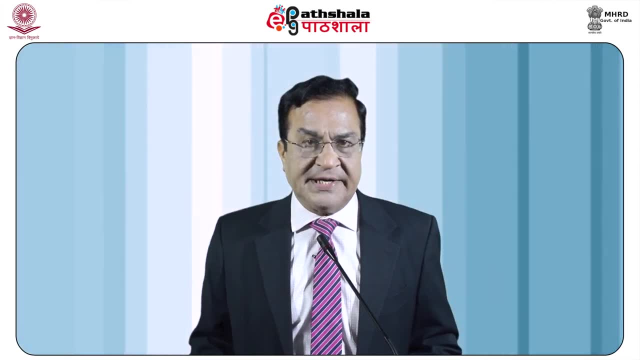 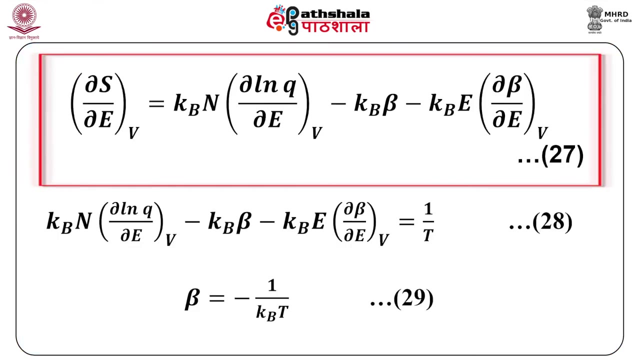 And the equation which we had got from statistical mechanics. if you remember that equation 22, if we differentiate it with respect to E at constant volume, then we get this: as you can see here, delta S by delta E at constant volume gives kB N, delta ln Q by delta E at constant. 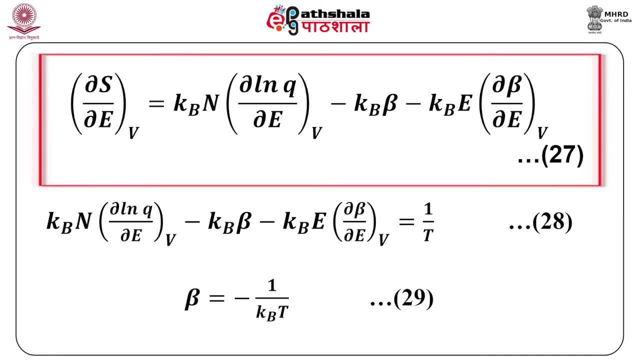 volume minus kB E delta beta by delta E V. And if we equate these two equations- 26 and 27- one is coming from statistical and the other is coming from classical thermodynamics- we get this: kB N is equal to delta ln Q by delta E at constant volume. minus kB beta is minus kB E delta beta by delta E at constant. 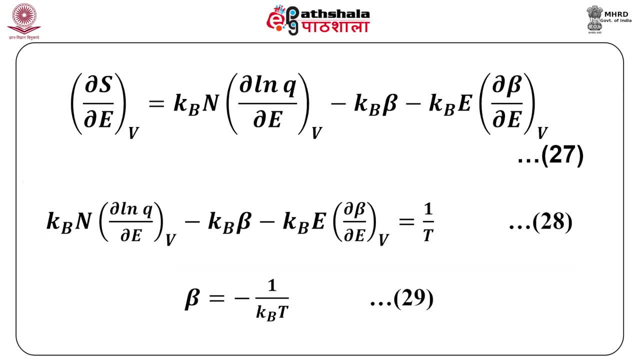 volume is equal to 1 upon T. This we will show later- that in the left hand side, First term and the third term, they are equal and they ultimately cancel out. And once they cancel out, we will be left with the expression we have shown now that beta. 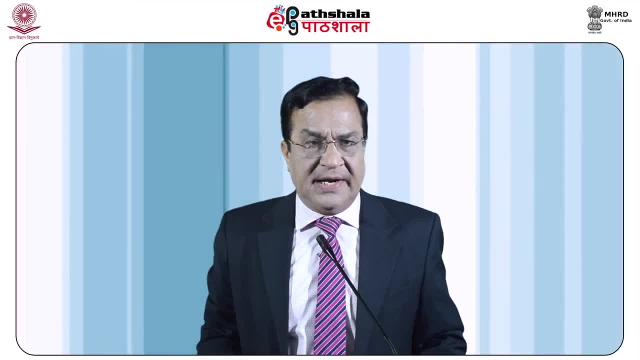 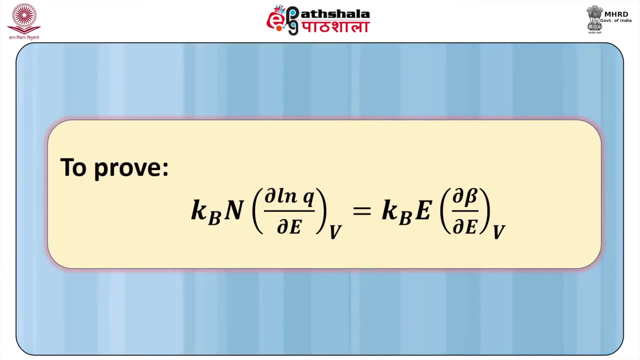 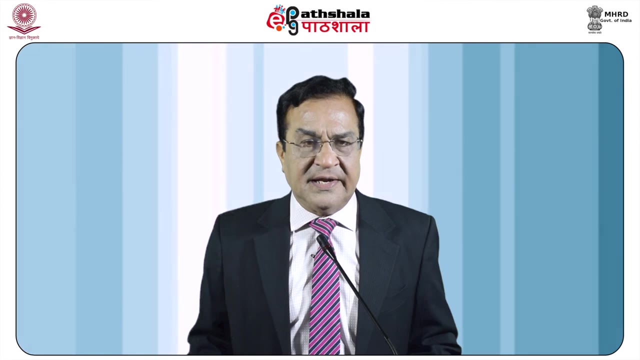 is equal to minus 1 upon kB by T, And in this we assume that this will be so only if kB N delta ln Q by delta E V is equal to kB E delta beta by delta E V. If we look at left hand side, we can expand it little bit, as you can see, left hand side. 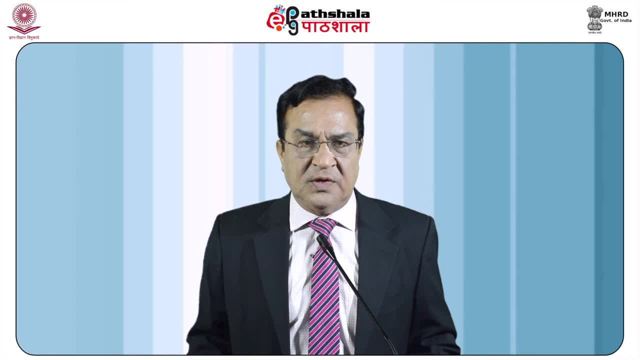 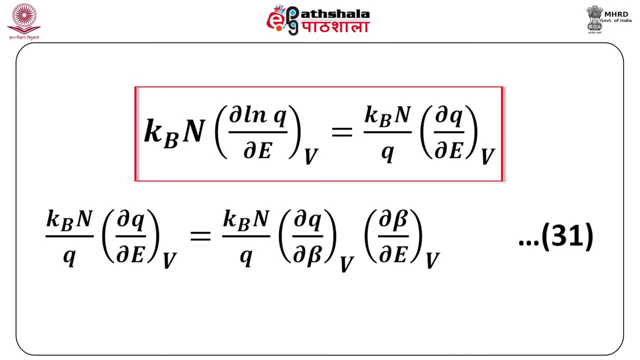 we can take differential of ln Q, it will become 1 upon Q. So we will be left with kB N delta. ln Q by delta E at constant volume is equal to kB N upon Q. delta Q by delta E at constant volume And if we simplify it further, divided by Q. 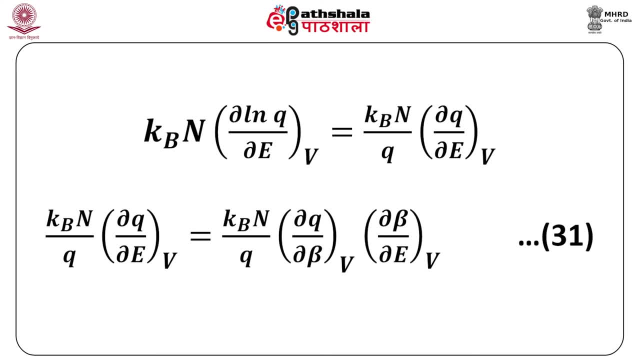 On both sides. you can see here we ultimately get this equation: kB N upon Q, delta Q by delta E at constant volume can be written in this way, that is, kB N by Q, delta Q by delta beta at constant volume, and then delta beta by delta E at constant volume. 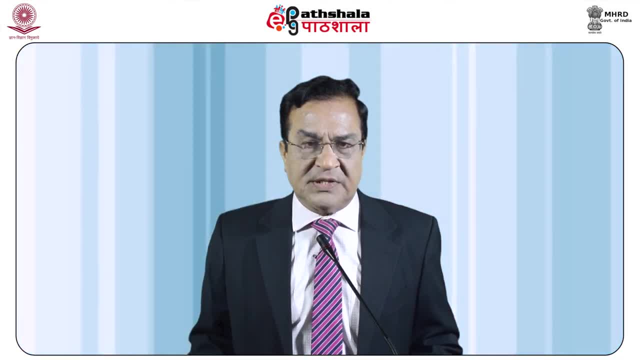 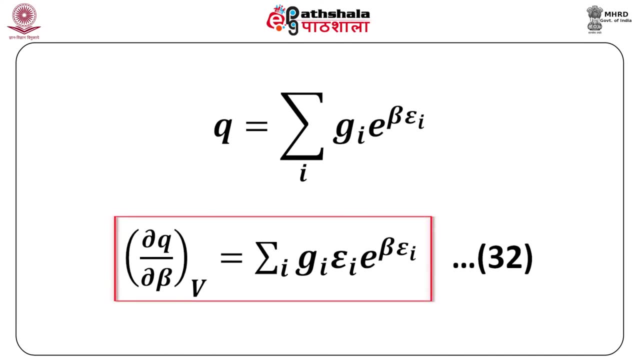 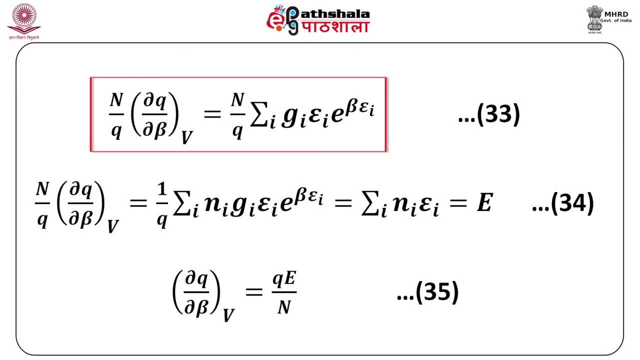 So from this equation, since we know that Q is equal to this, this is the definition of the partition function. And if we here also take delta Q by delta beta, at constant volume, we get this. and then, multiplying by N, by Q, ultimately we get this relation where you can see that ultimately, 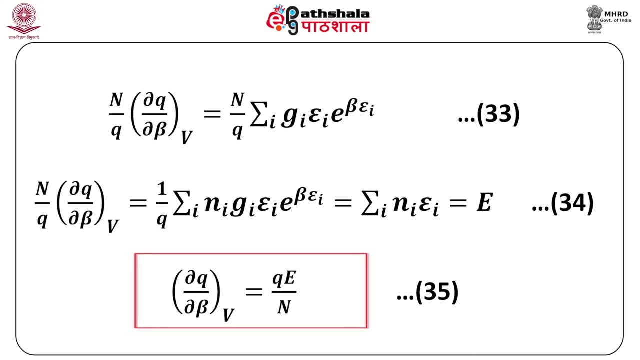 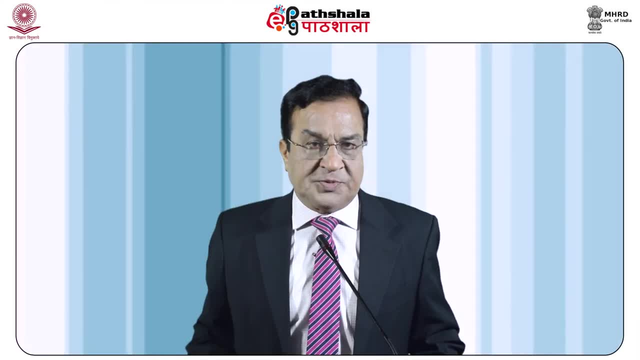 the whole solution gives delta Q by delta beta at constant volume is equal to Q? E by N. that is the equation 35.. Substituting equation 35 in equation 35.. So we can see that delta Q by delta beta at constant volume is equal to qE by N, that is. 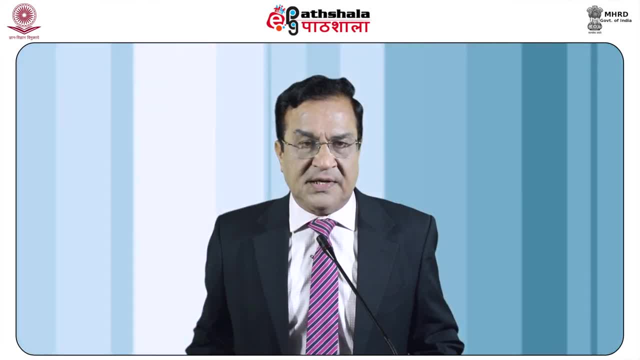 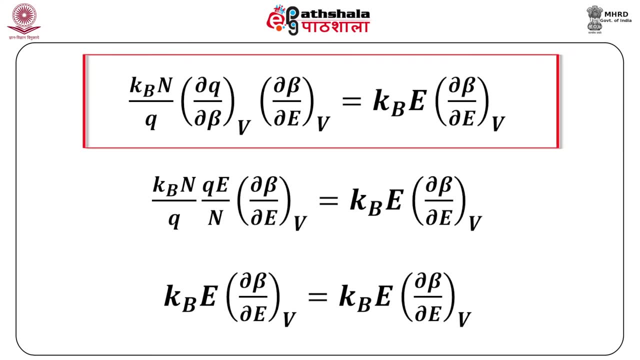 the equation 35. So this equation 30 gives, as you can see here, kB N by Q delta Q by delta beta V. delta beta by delta E V is equal to kB E delta beta by delta E V. Whether these two are equal or not, this has been shown here very explicitly. 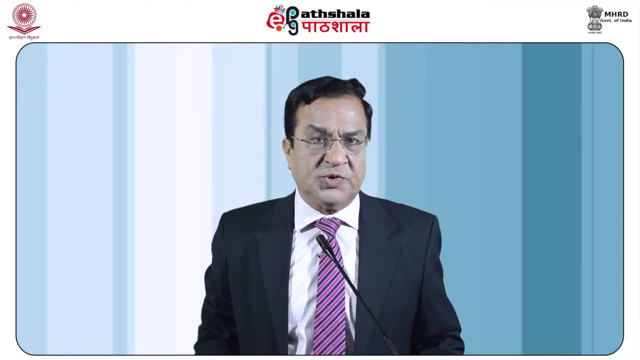 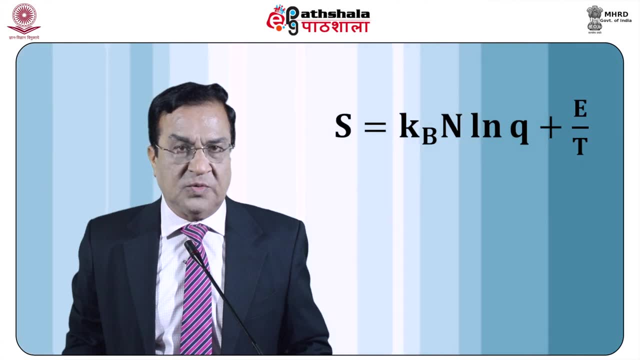 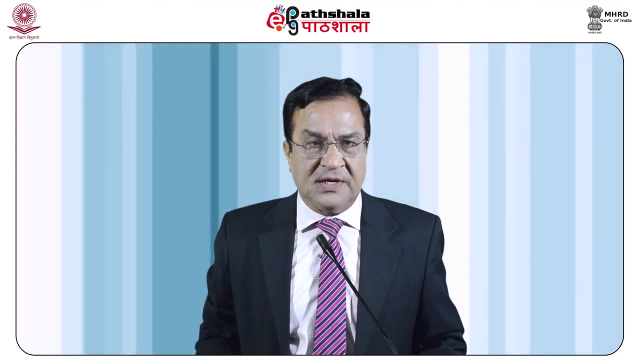 After having done this now, and if we substitute the value of the beta now we get the expression for entropy, Which is: S is equal to delta Q by delta E V. S is equal to kB, N, ln, Q plus E by T. So this is a very important relation where entropy 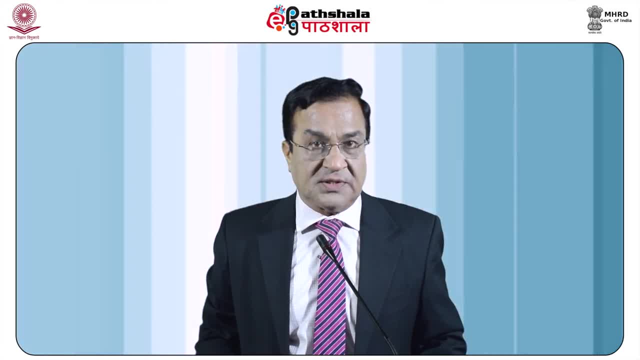 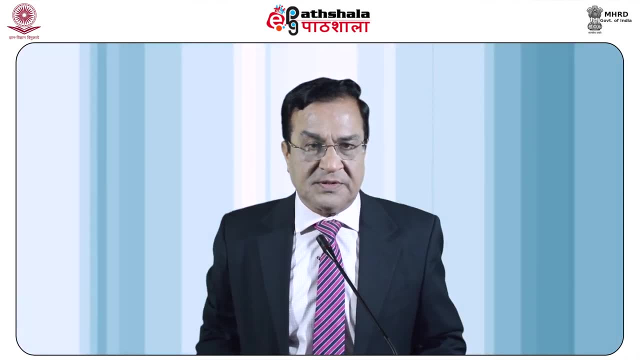 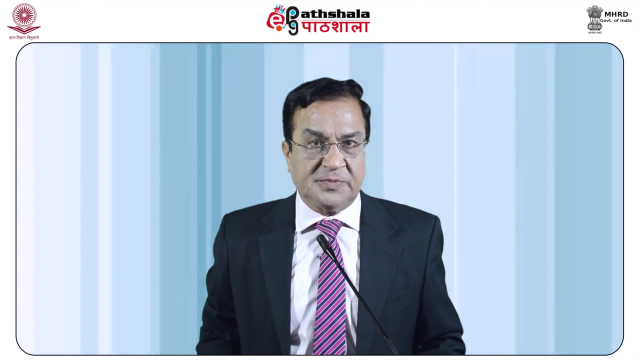 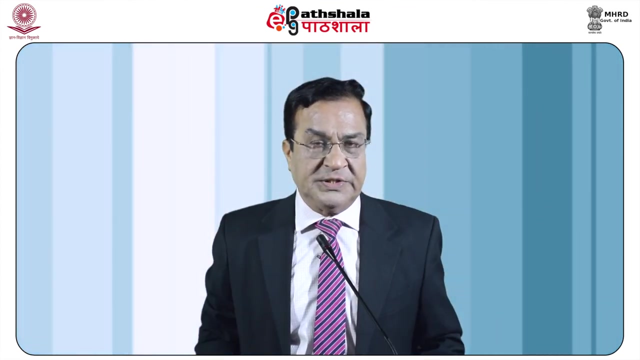 has been related to partition function. So this is a equation which will be of great use in the subsequent modules. So in this module today we have studied about the Boltzmann equation. where S is equal to kB, ln, W, We have shown that the W, which is the thermodynamic probability, it corresponds. 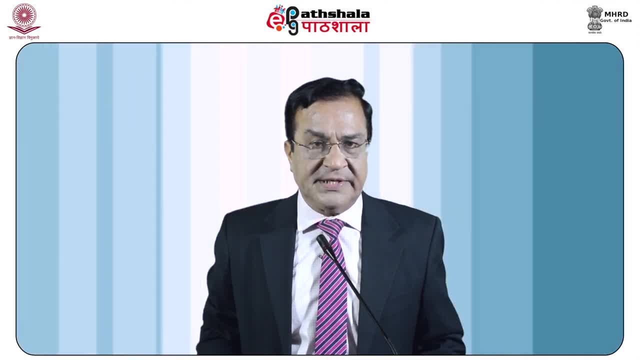 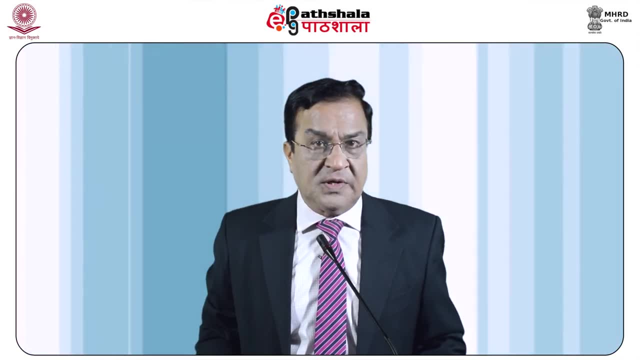 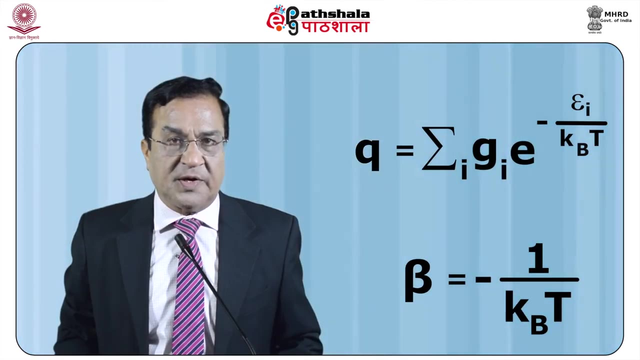 to the most probable macrostate. That is what we did, and then we said that this equation will apply to all systems. We have also derived the expression for the beta and we have shown that beta comes out to be equal to minus 1 upon kB T And therefore the expression for the partition function. 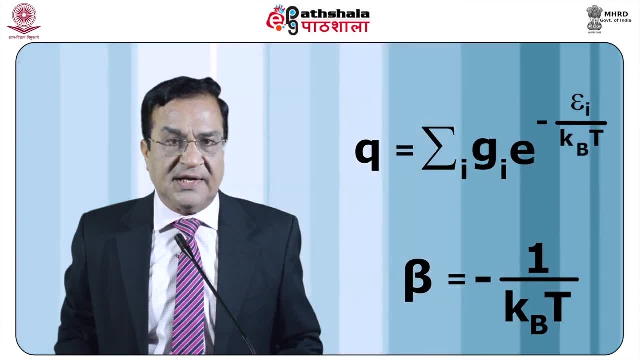 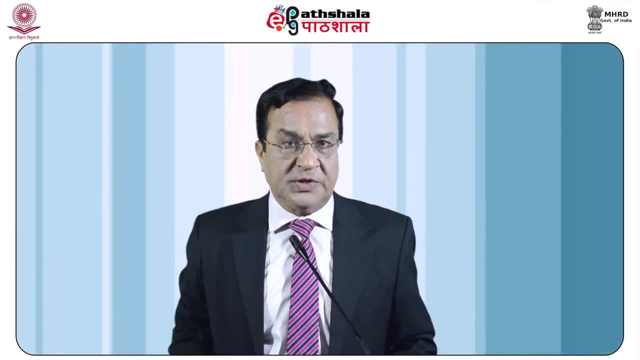 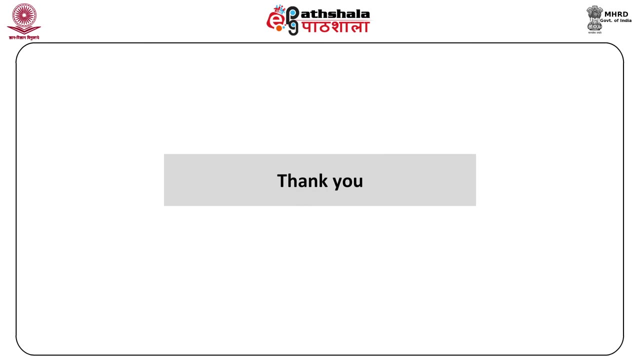 becomes, Q is equal to summation i Gi e to the power minus epsilon i by kT. And then, lastly, we showed that entropy S is related to partition function. So this is a very interesting expression to be used for the third-party equations. So let's take a look at it. So we are going to use the first equation. So the first question is: what is the temperature of the second-party equation? And this is going to be the first question of the third-party equation. Let's take a look at the first question.